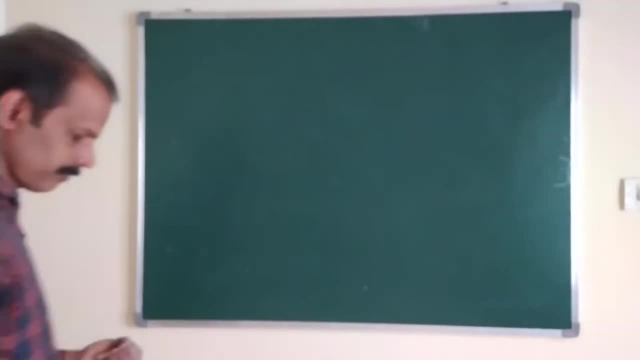 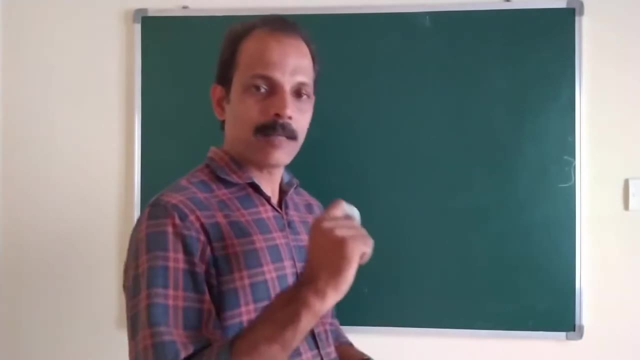 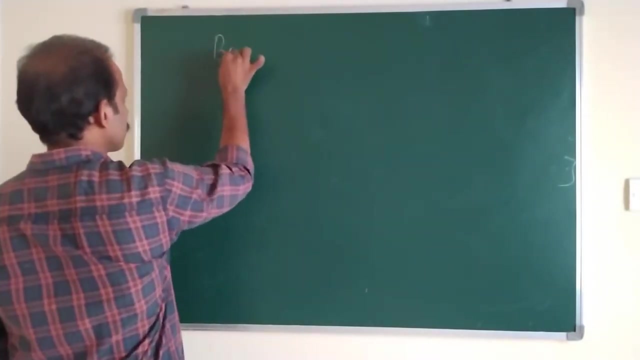 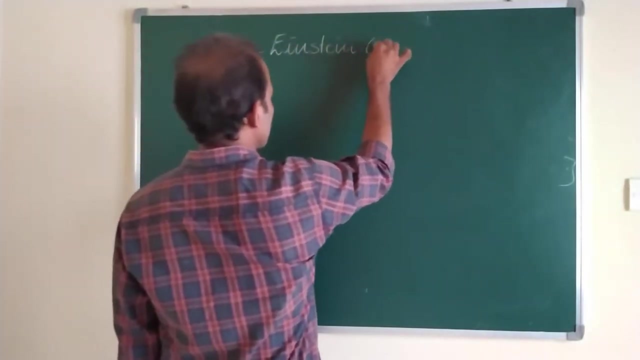 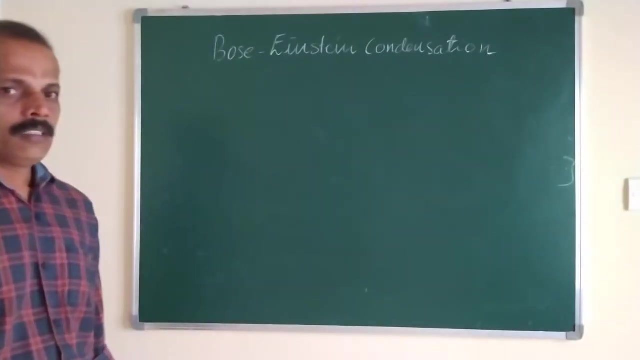 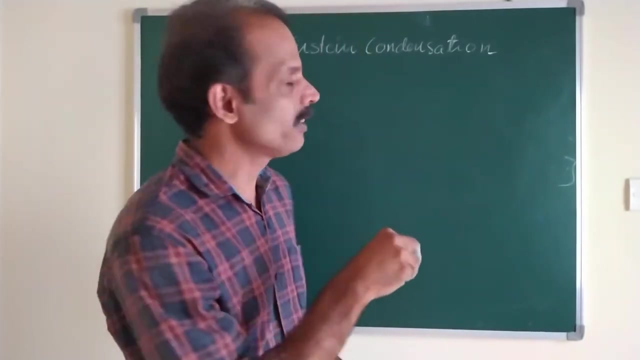 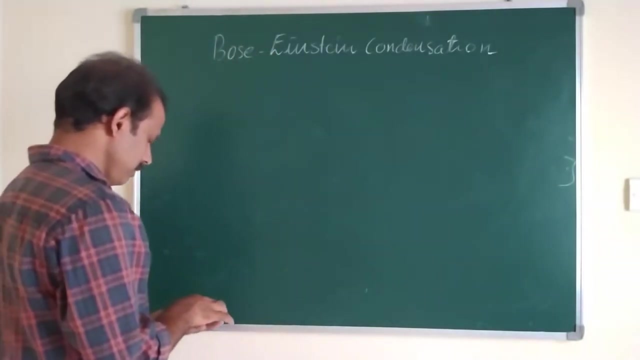 Hi everyone, welcome back. Today we are discussing ideal Bose gas and Bose-Einstein condensation. What is a Bose gas? Bose gas or Bose volts, They are the particles which obey Bose-Einstein statistics, That is, with the integral spin, particles with the integral spin, So you. 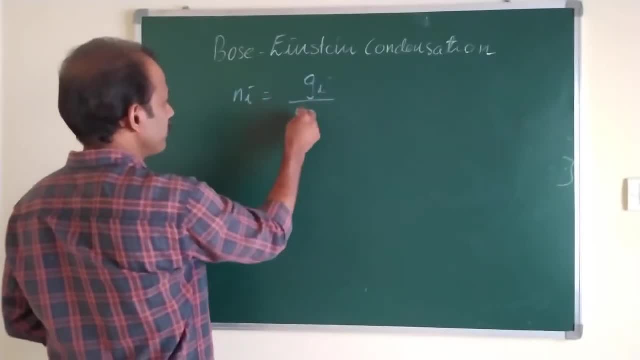 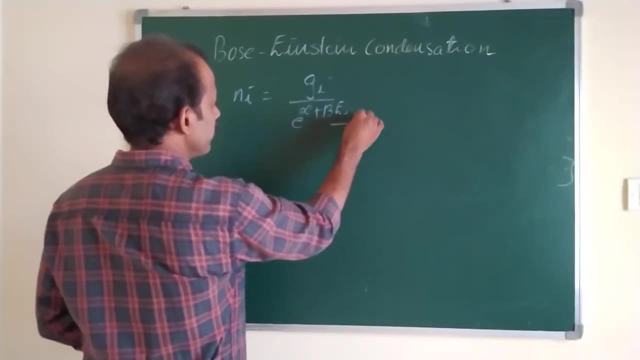 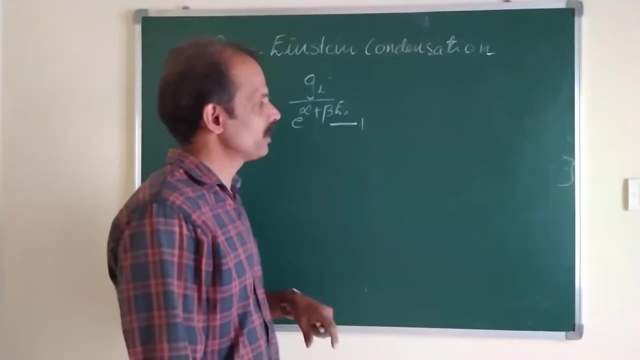 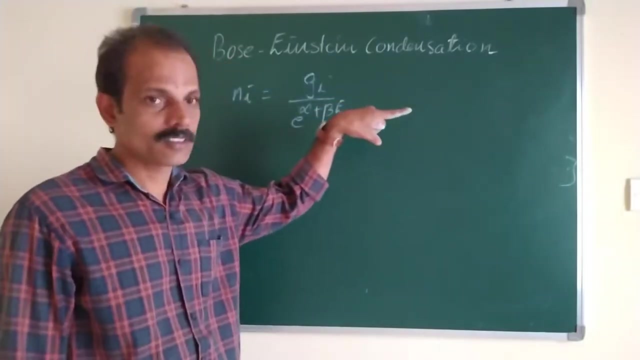 know n, i is equal to g a divided by a raised to alpha plus beta plus beta plus beta plus e i minus 1.. That is the distribution. That is the distribution. And any particle which obeys the statistics is known as Bose bosons or ideal Bose gas. And when we take the summation, 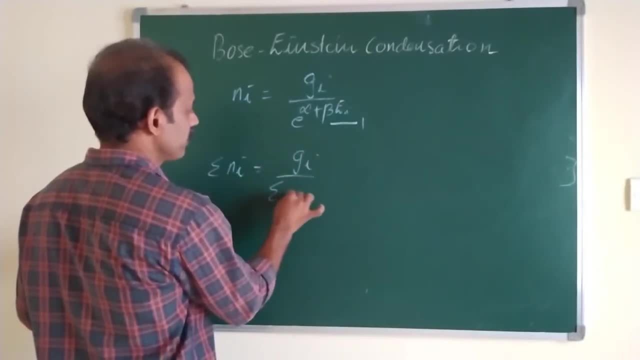 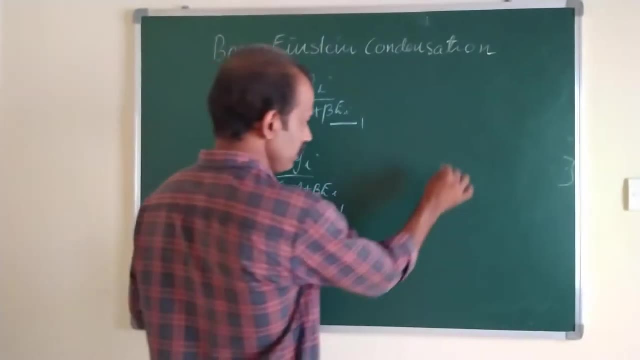 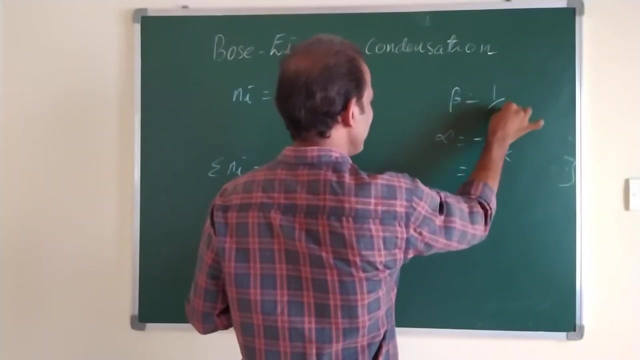 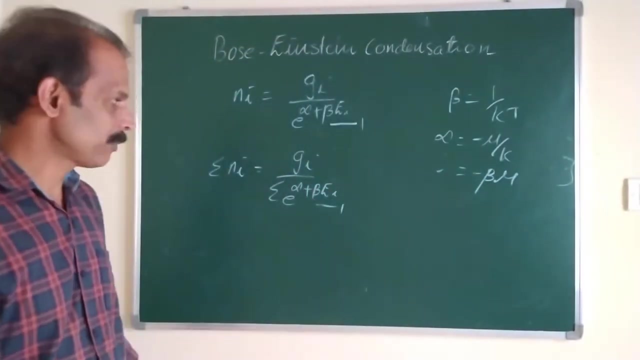 we get g a divided by sigma e, raised to alpha plus beta of e i minus 1.. But alpha is equal to minus mu by kb. This is equal to beta is equal to 1 by kb. So alpha is equal to minus beta mu, Where mu is the chemical potential. So we can replace. 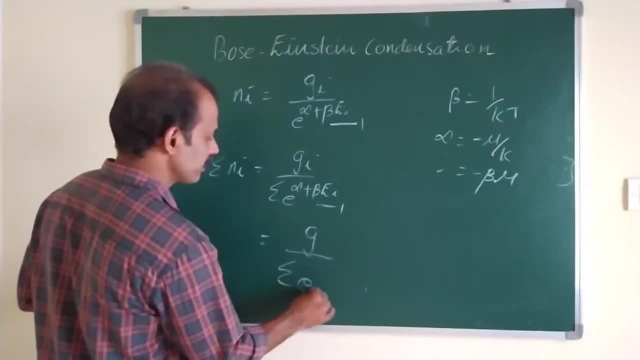 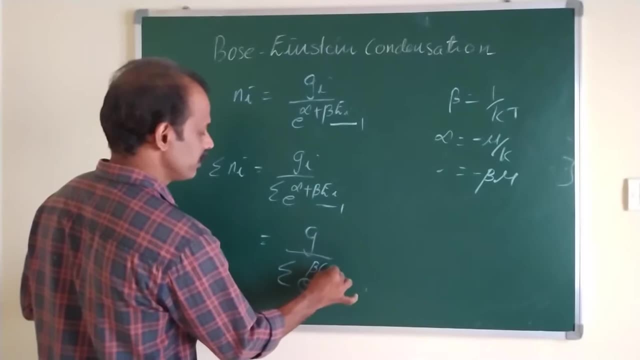 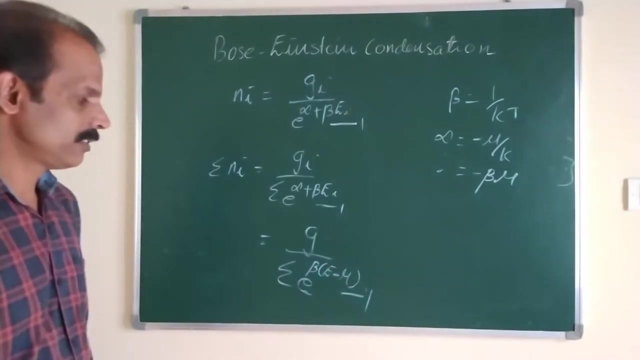 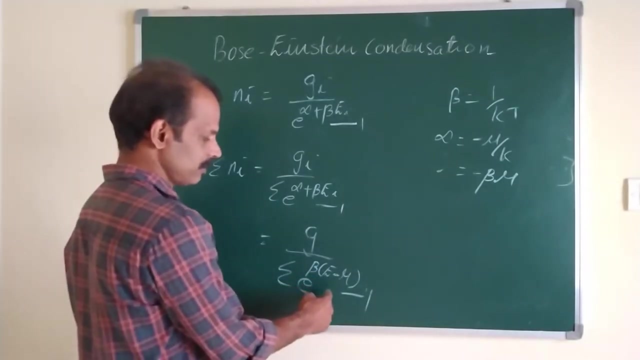 it as g divided by sigma e raised to minus beta. or we can say beta into a minus mu. So e i is equal to g to the power minus mu into g to the power minus 1.. What does this mean? It means that e to the power minus mu is equal to g to the power minus. 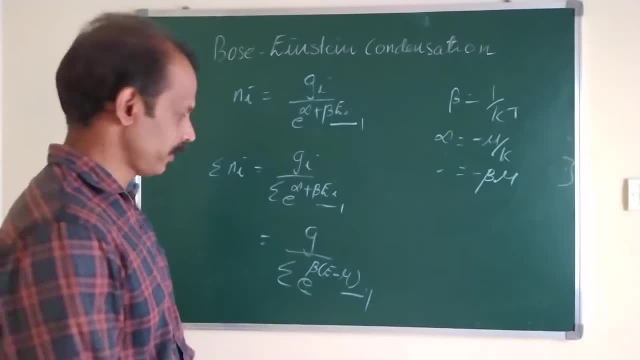 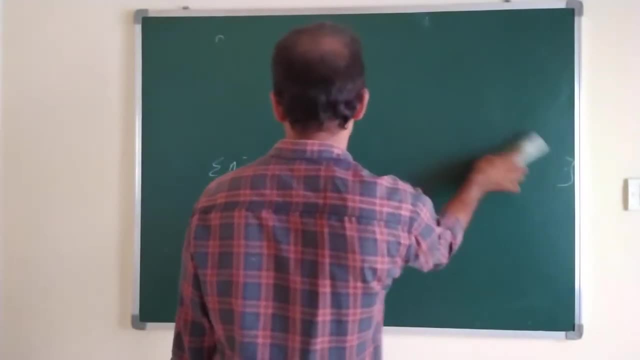 1. That is the equation. So the expansion, And in this situation there is a big difference. that is, it is the expansion of gamma, which is minus g to the power, minus mu. There is a big difference. So we will explain that. 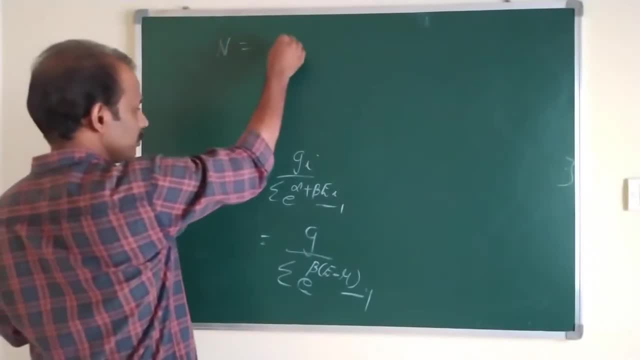 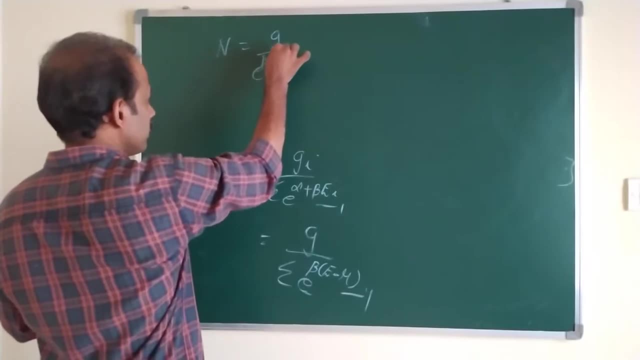 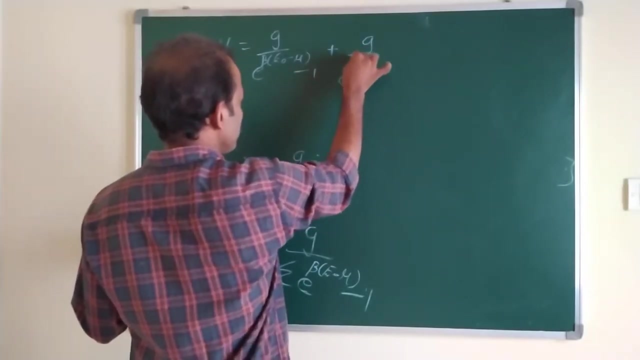 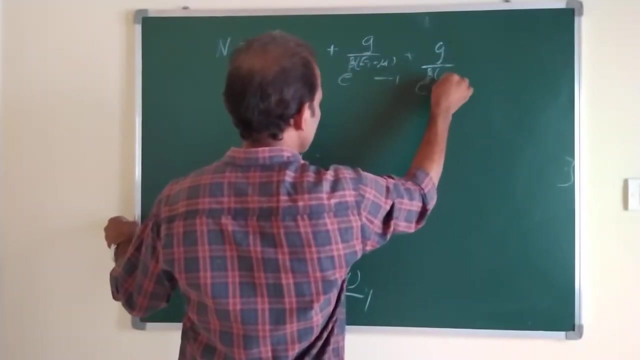 G to the power minus mu. So that is the equation: n. i is equal to g by e raised to beta, e to the minus mu minus 1 plus g, by e raised to beta into e1 minus mu minus 1 plus g, e raised to beta, e to the minus mu minus 1 plus plus plus plus 1.. 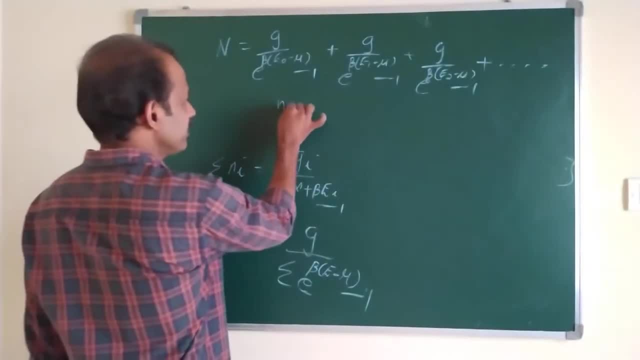 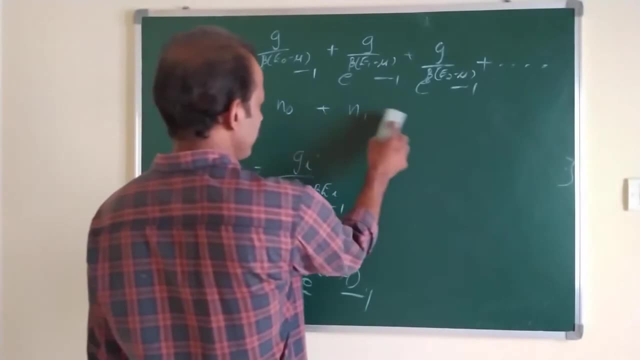 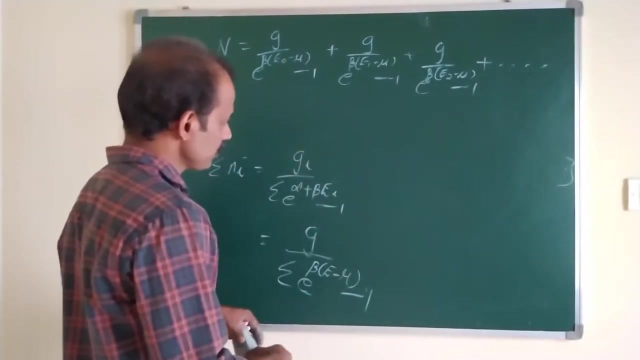 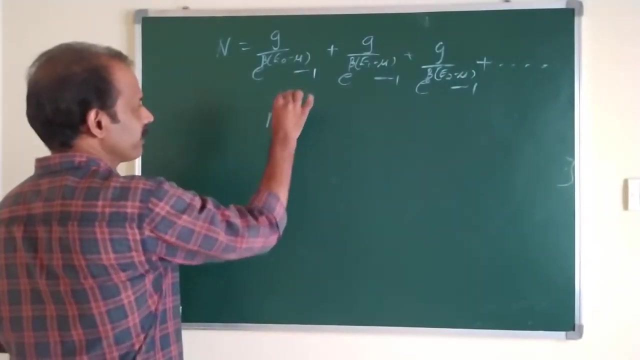 So and so That is, it is n0 plus n1 plus n2 and so and so We have seen this separation earlier. Okay, Here the number of particles, that is n. i never be 0 or never be negative. 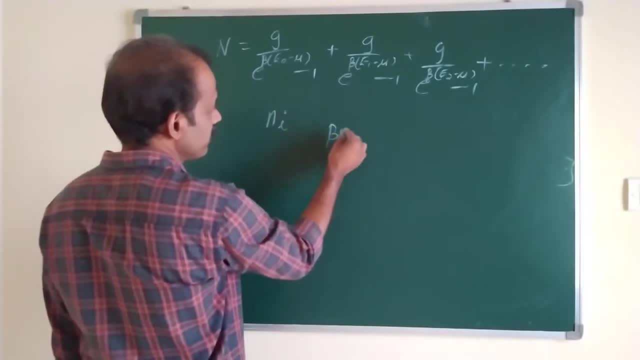 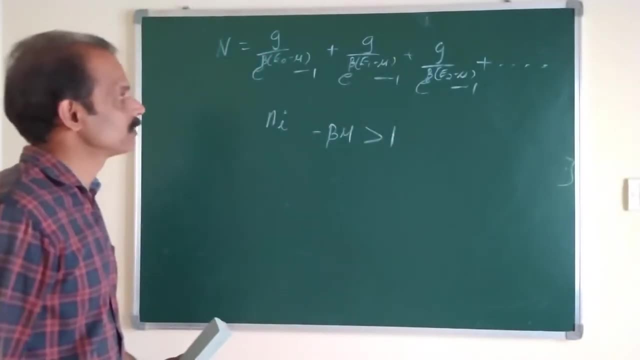 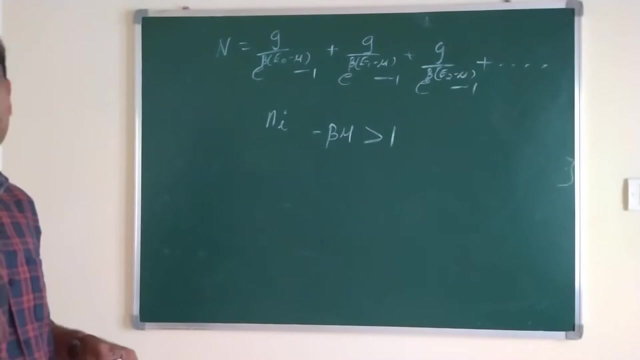 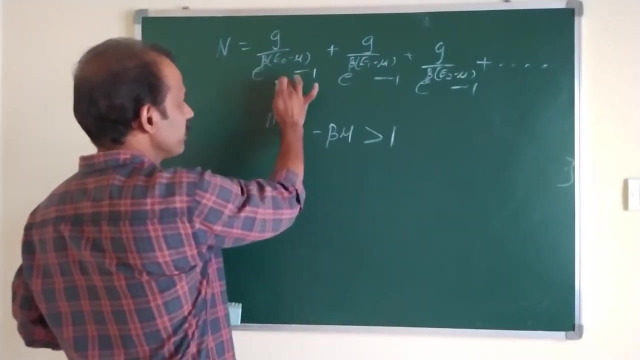 So this term, That is, beta or minus beta u, should be greater than 1.. b0 minus or beta e i minus beta mu, So minus beta mu should be greater than 1.. Then how do we get a value here? 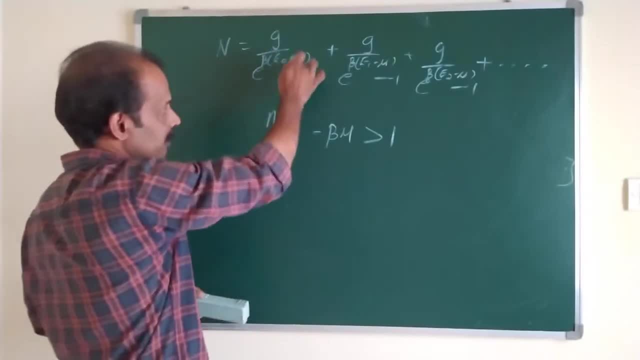 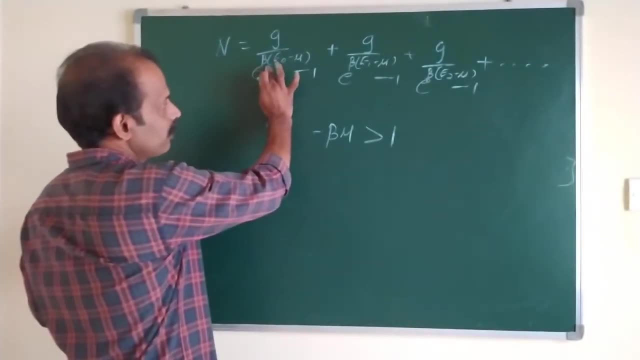 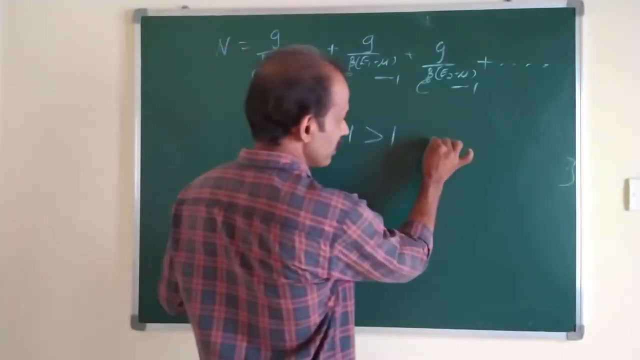 Then dividing that by- sorry, that term, Degeneracy is divided by the term- We should get a positive value. So minus beta, mu should be greater than 1.. That is, mu should be less than or equal to 0.. 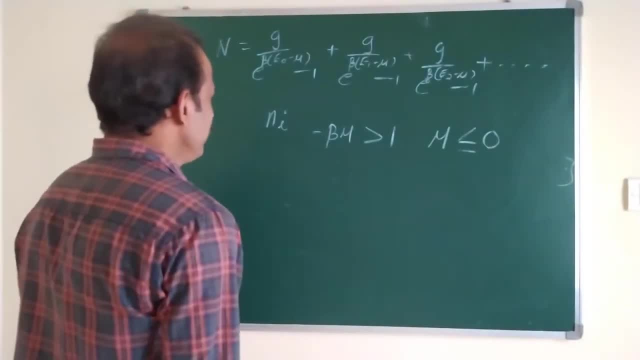 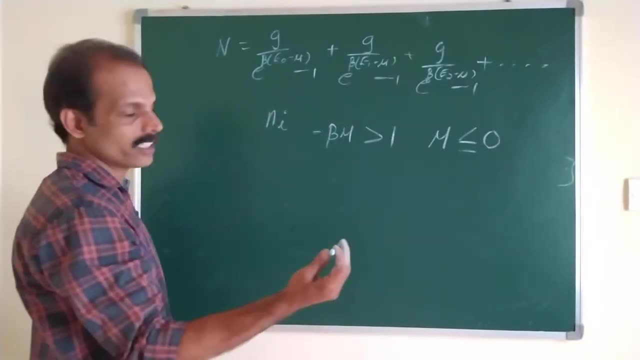 Less than or equal to. That is our assumption. Okay, There is a consequence here: When mu is equal to 0, e0, you know the ground set energy, e0 is equal to 0. And mu is equal to 0. 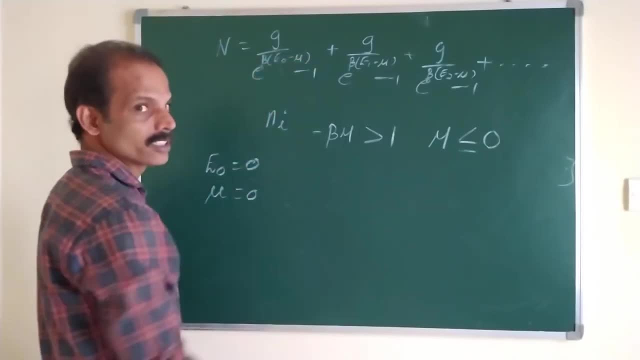 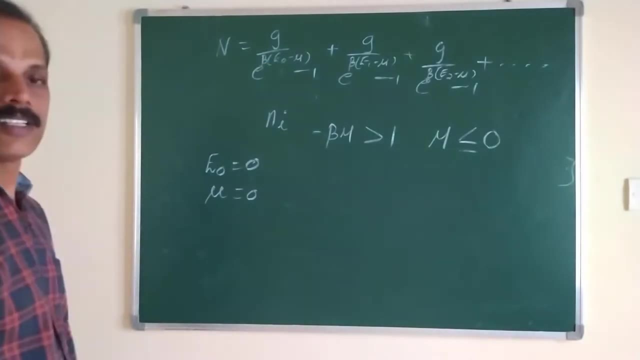 Then e raised to b, beta into 0. That is e raised to 0.. e raised to 0 is 1.. 1 minus 1 is equal to 0. That is g divided by 0. So that term will vanish. 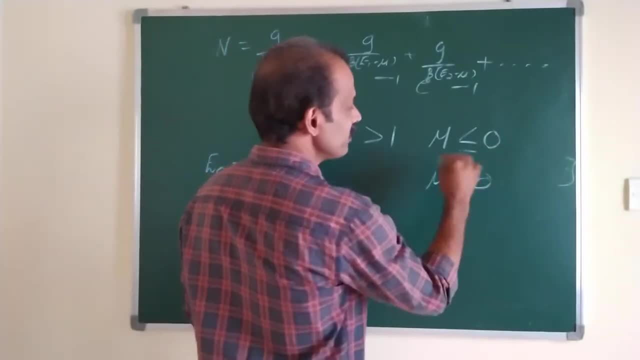 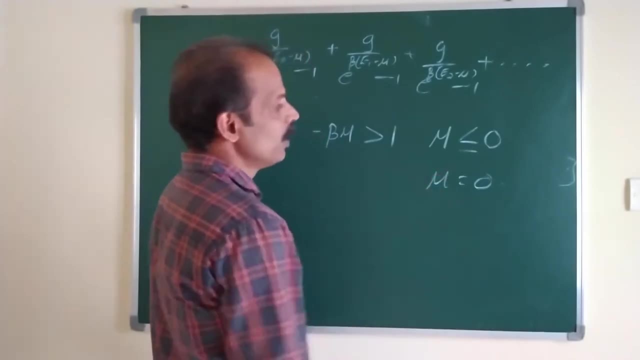 So at maximum value. the maximum value of mu is 0.. Next value is negative value. Less than 1.. Less than 0.. Less than 0. So the maximum value of mu is 0.. At the maximum value, this term vanishes. 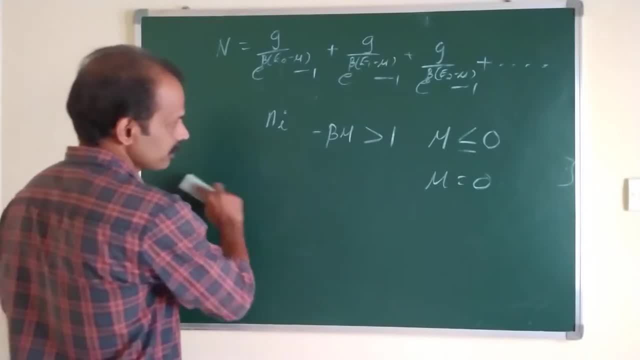 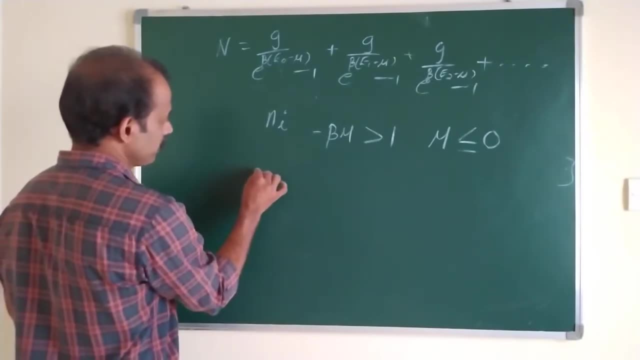 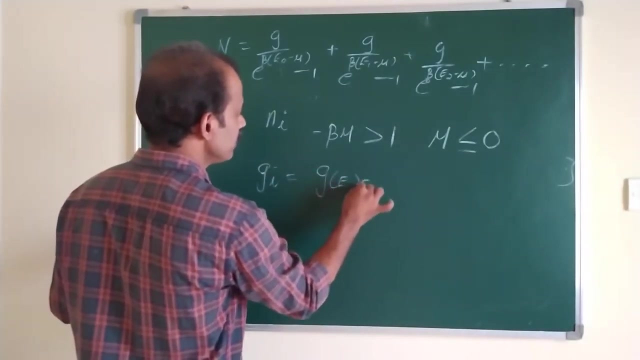 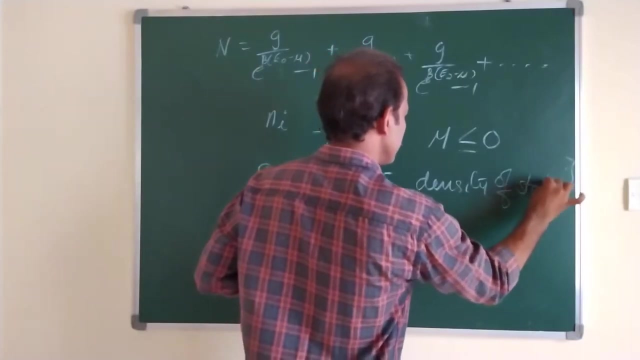 Okay, We will discuss it later. Then we are converting this into integration, Because g i, which is equal to g e, into d And it is known as density of states. Density, Density of state, The standard value of g e d. 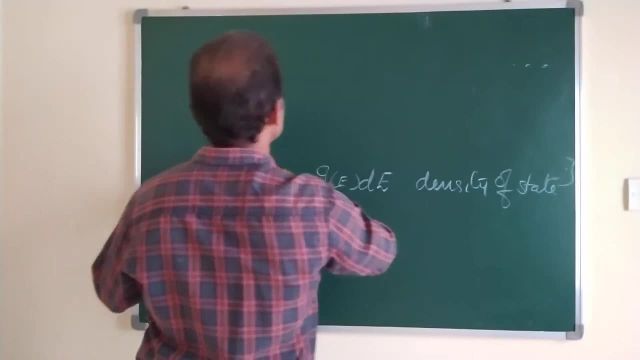 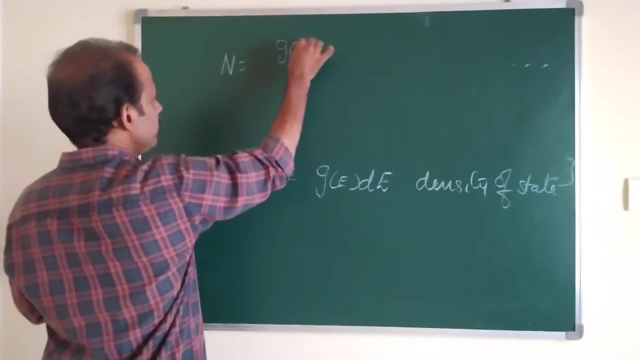 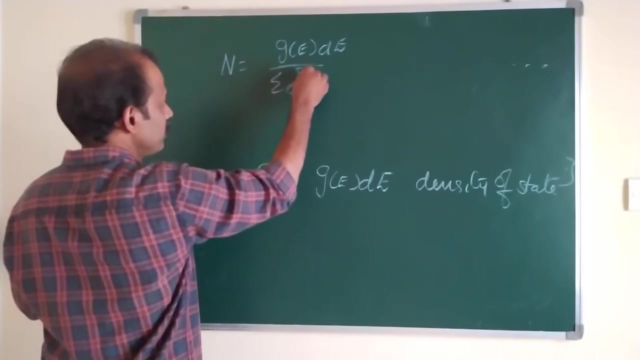 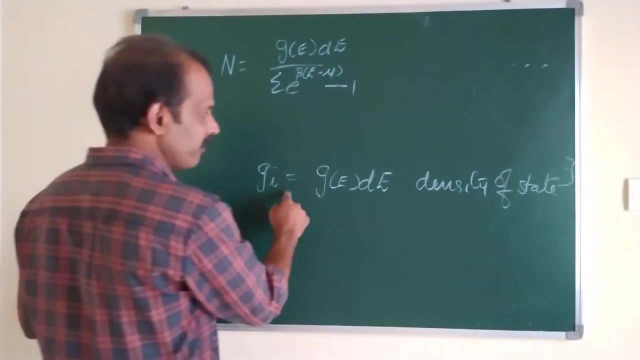 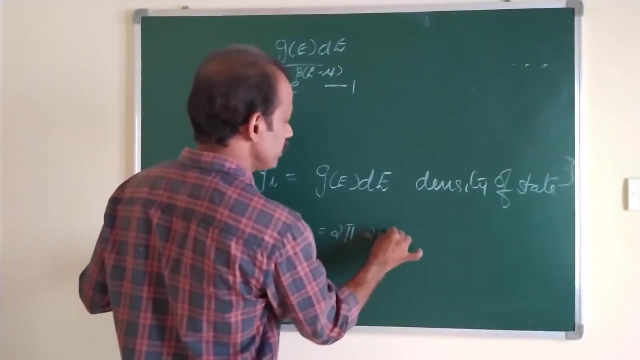 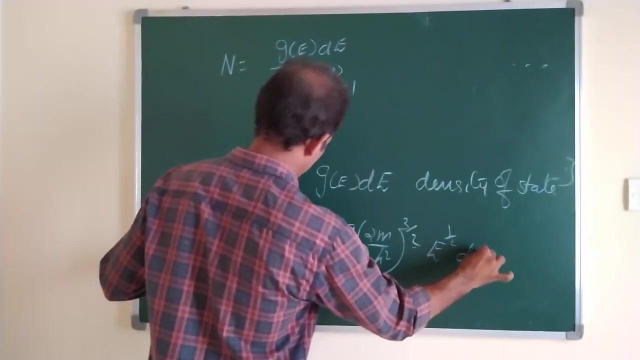 That is, we can replace the equation That is n equal to g e into d e divided by sigma, e raised to beta, into e, i minus mu minus 1.. Okay, And the standard value of this g e, that is density of state, which is equal to 2 pi into 2 m, by h square over 2 raised to 3, by 2 into e, raised to half into d. 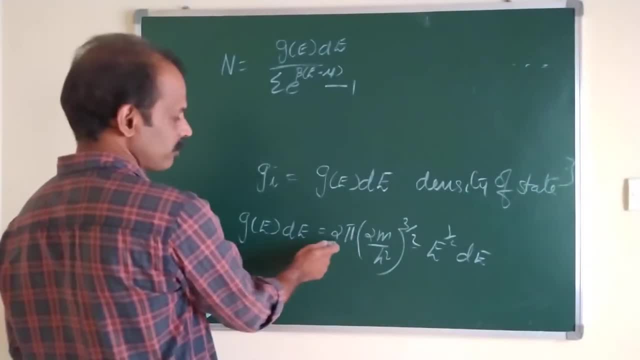 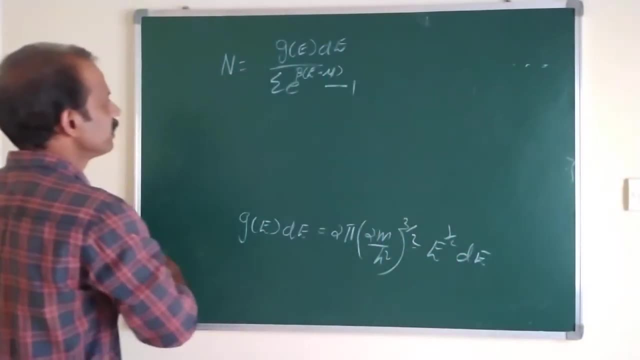 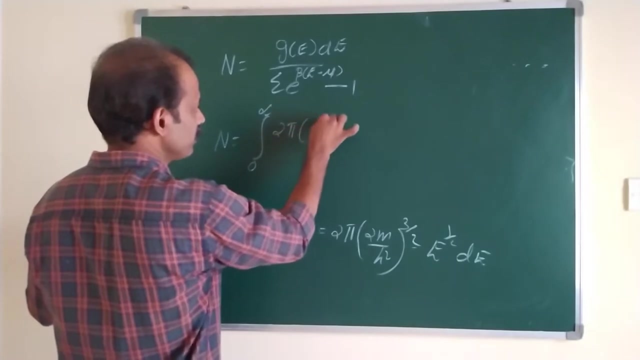 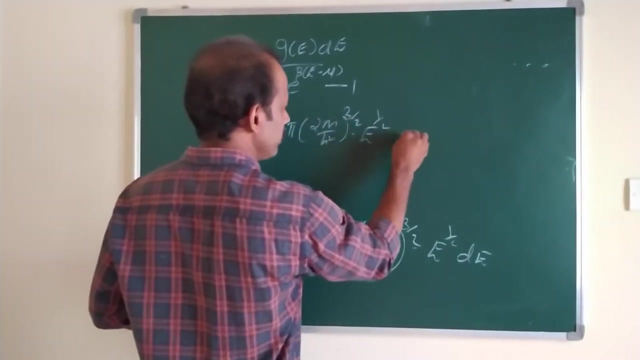 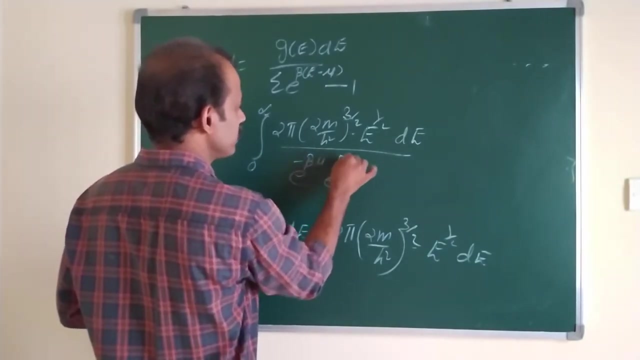 That is the standard value And we are substituting this value here and converting, That is, replacing summation by integration. We get: n is equal to Integral 0 to infinity. 2 pi into 2 m by h square over 2. raised to 3 by 2 into e. raised to 1 by 2 into d, e divided by e. raised to minus beta mu into e raised to beta e minus 1.. 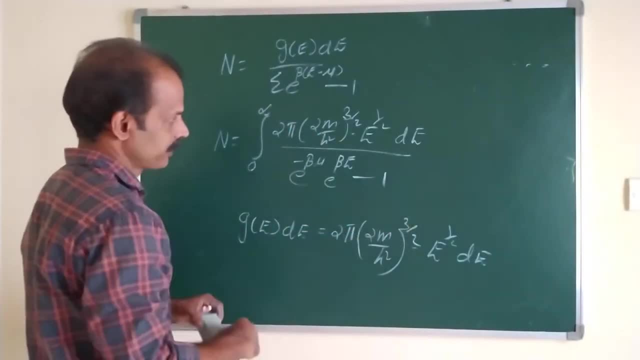 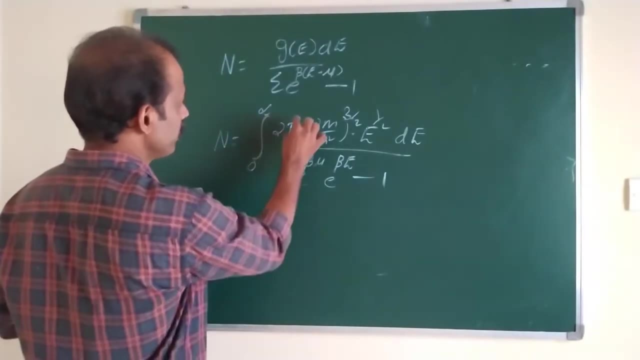 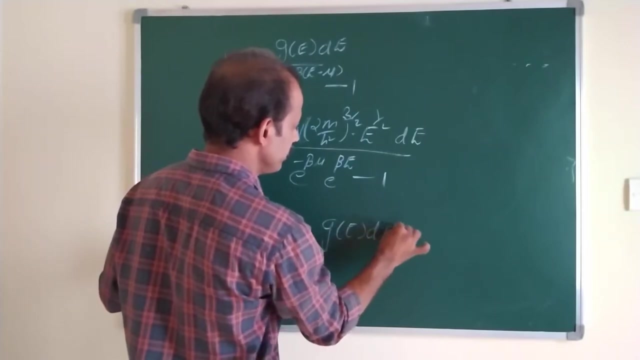 Okay, This term, This term we have asked, And then Taking the constants out, So we get 2 pi into. So there is a small mistake. That is g e into d e, Density of state. So value should be there. 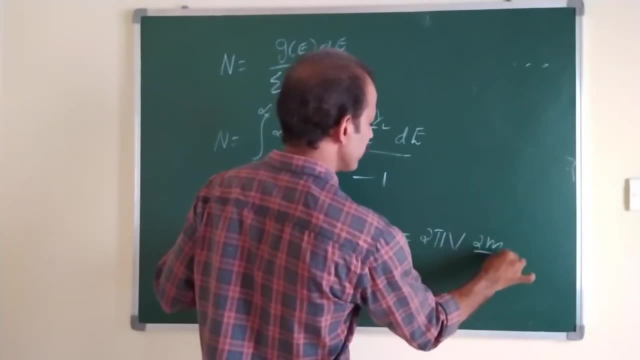 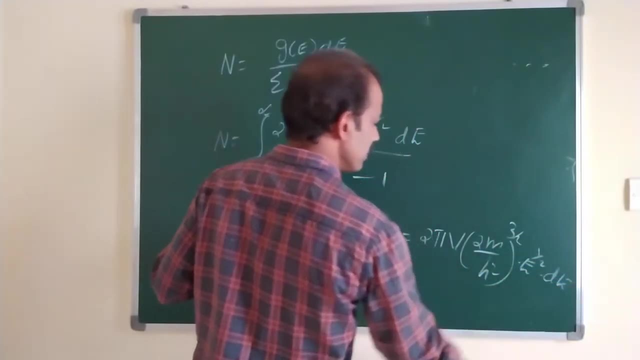 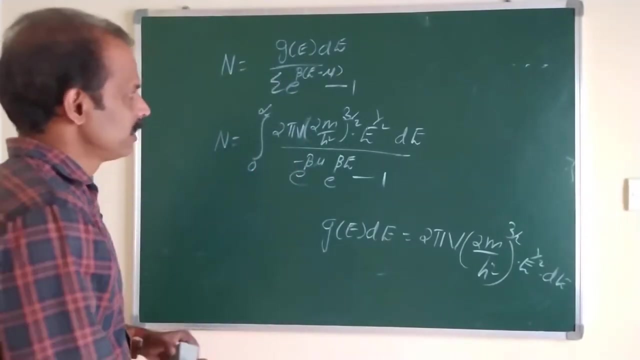 Which is equal to 2 pi into v into 2 m by h, square over 3 by 2 into e, raised to 1 by 2 into d e. Sorry for the omission. So there should be. So there should be a volume term here. 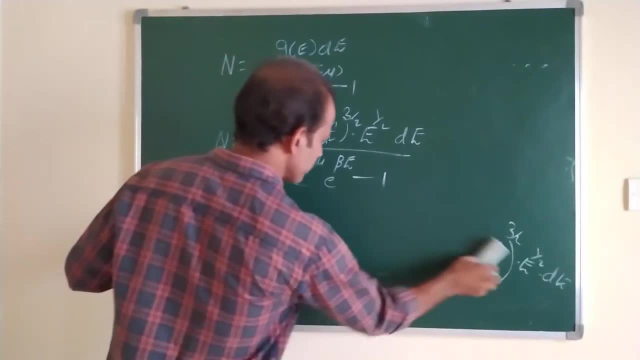 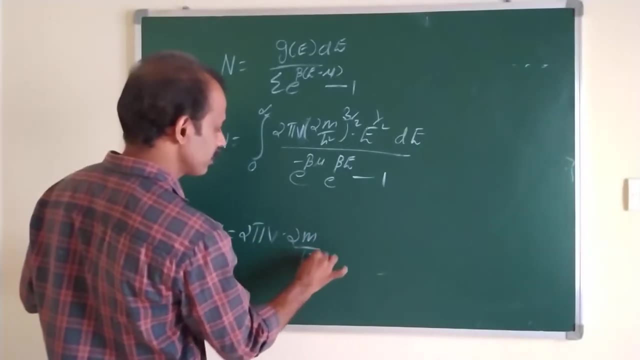 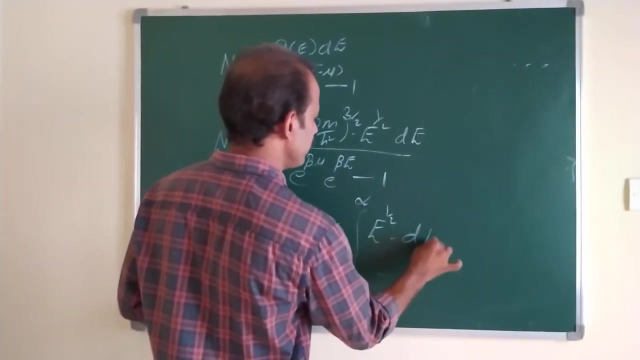 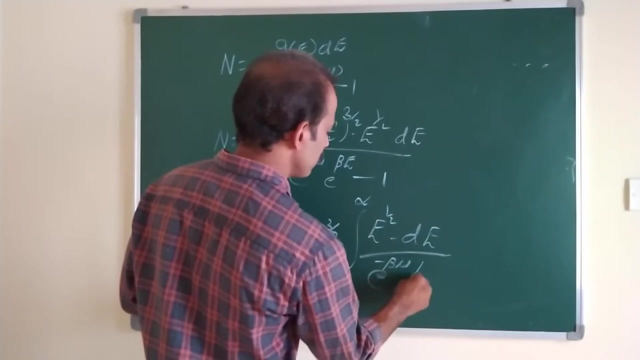 Okay, So we are taking the constants out. So we get n equal to 2 pi into v into 2 m by h, square over, raised to 3 by 2, into integral 0 to infinity. e raised to 1 by 2 into d. e divided by e raised to minus beta mu into e raised to beta e minus 1.. 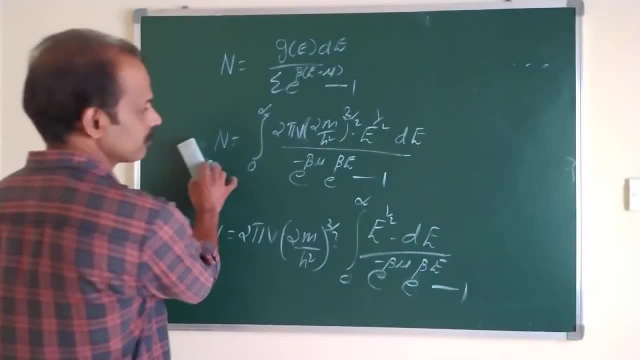 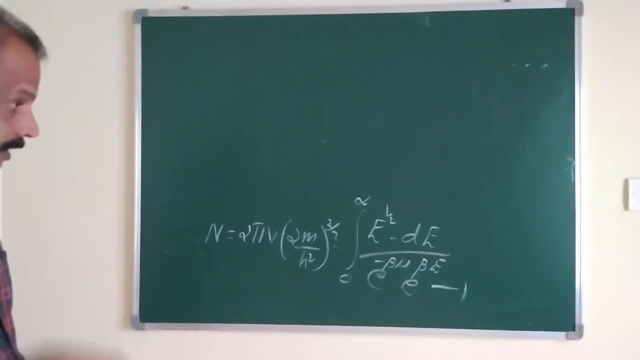 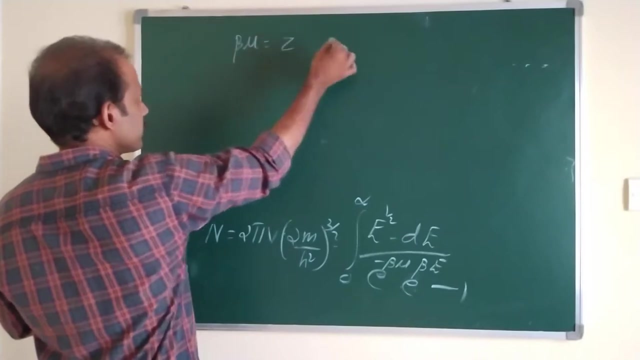 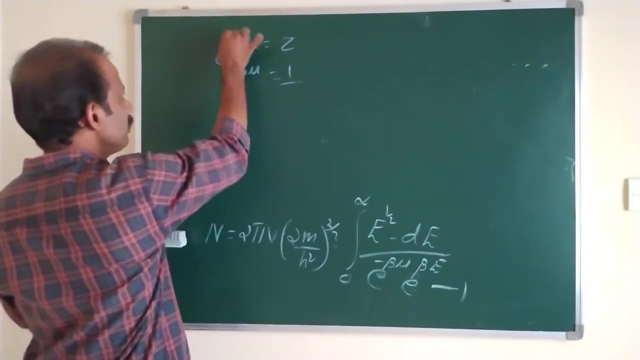 Okay, That is what we need. Alright, Now put: beta mu is equal to z. So e raised to minus beta mu is equal to Sorry. e raised to beta mu is equal to 1.. e raised to minus beta mu is equal to z. 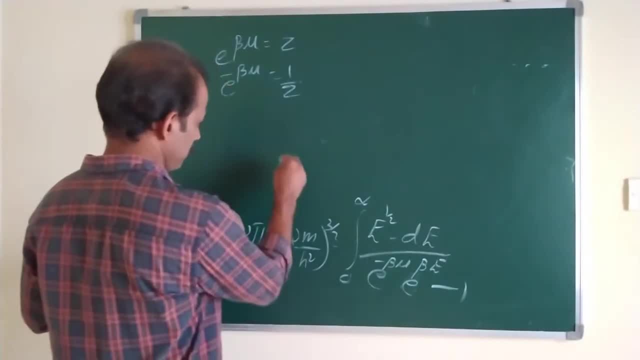 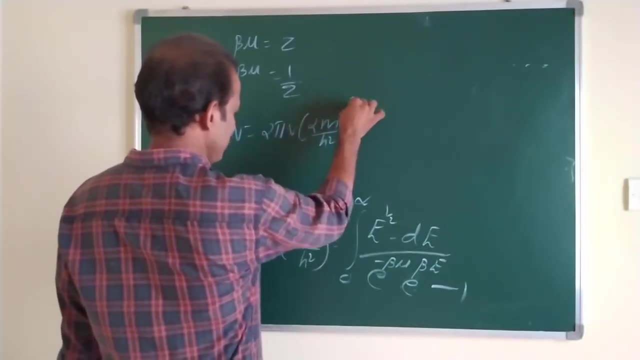 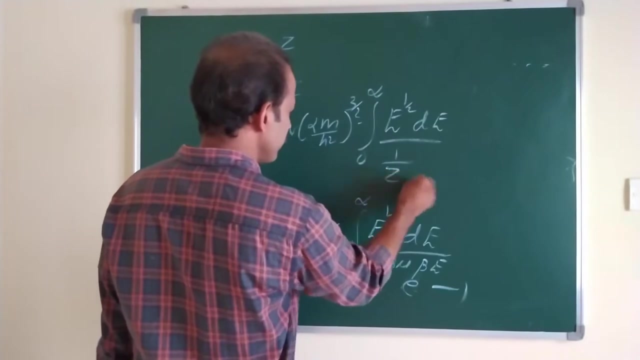 So. So our equation will become n equal to 2, pi will be 2m by s power, 3 by 2 will be integral, 0 to infinity. e raise to half, 2 into d, e squared by 1 by z into e raise to beta. e minus 1.. 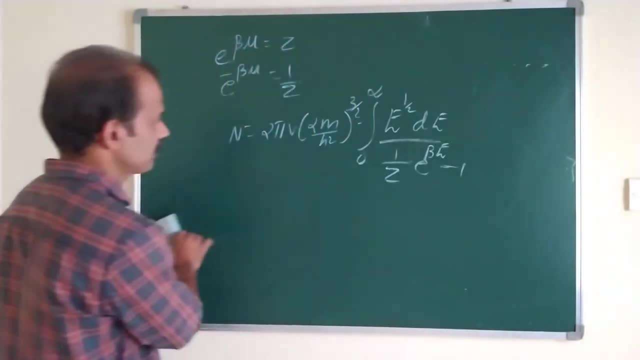 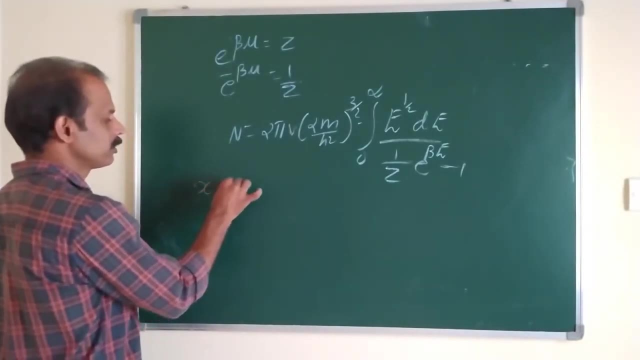 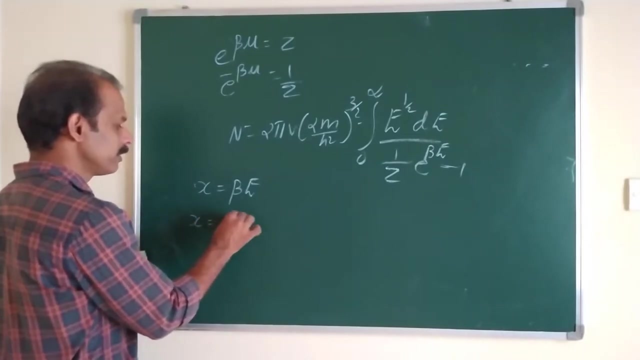 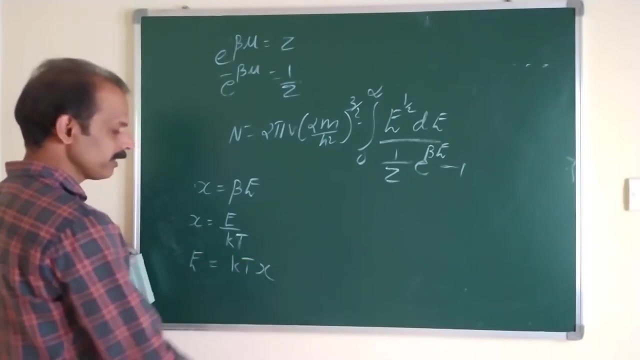 Again put dimension factor, that is term. so say x, which is equal to beta, e, d raise to 1 by kt. that is x is equal to t by kt, or e is equal to kt into x, d, e is equal to kt. 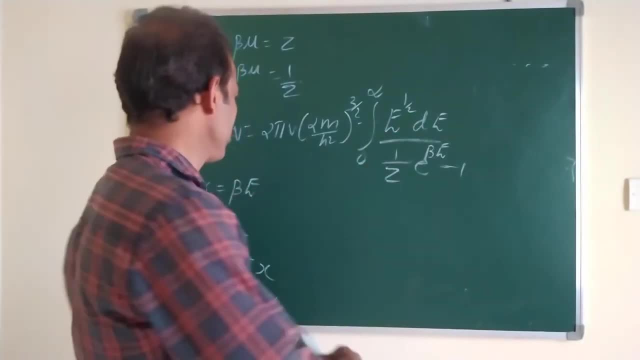 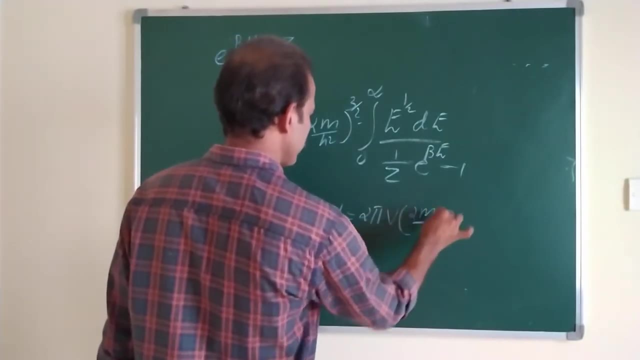 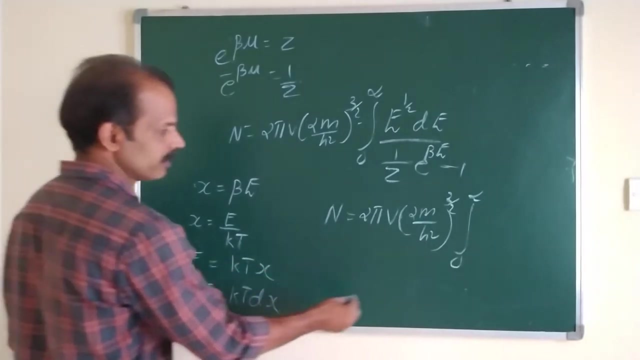 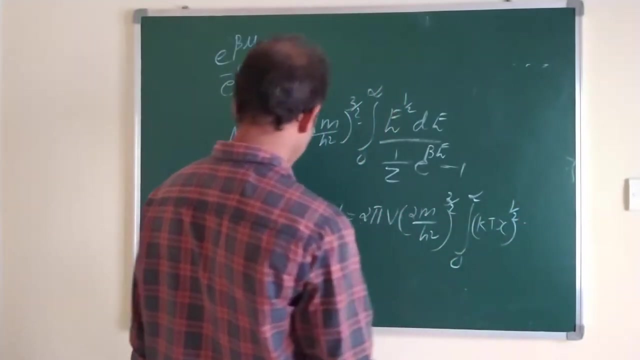 bx. Substitute these values here so we get n equal to 2, pi b into 2m by s power. all rise to 3 by 2 will be integral. 0 to infinity e raise to half, which is equal to kt x. all rise to half into d e. 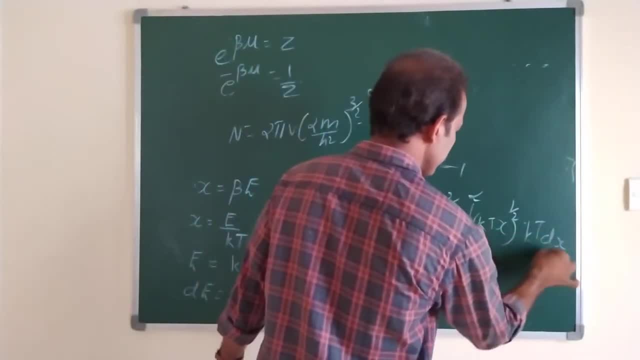 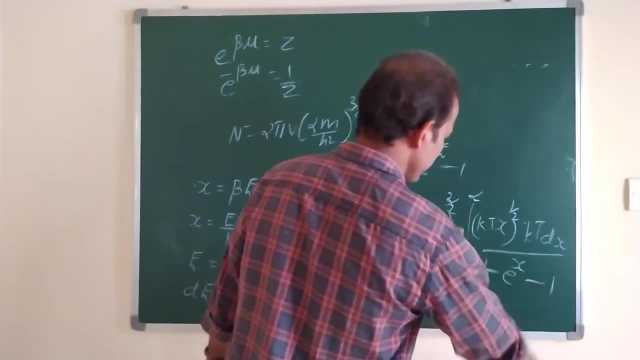 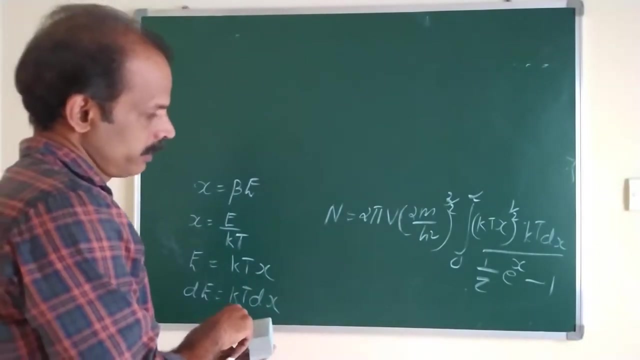 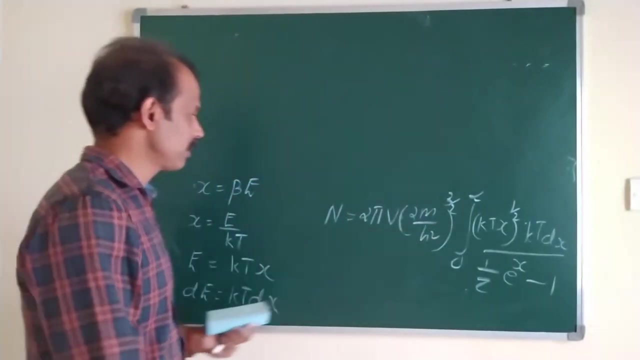 d. e is equal to kt. dx Divided by 1 by z, b is equal to x minus 1.. Then kt rise to 1 by 2 into kt. kt rise to 3 by 2, we are also taking this out, so our equation will become: n is equal to 2, pi into b, into 2m by s power. 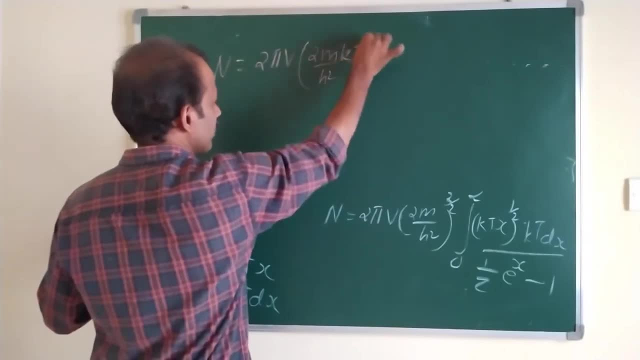 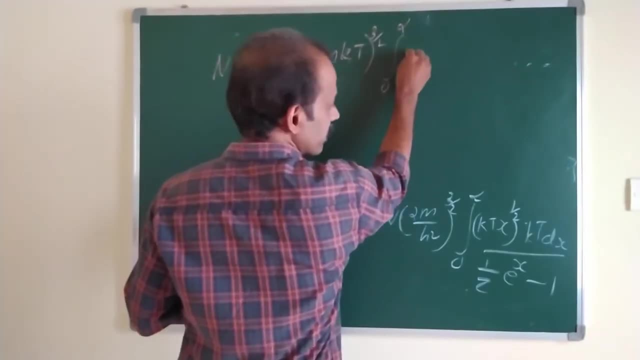 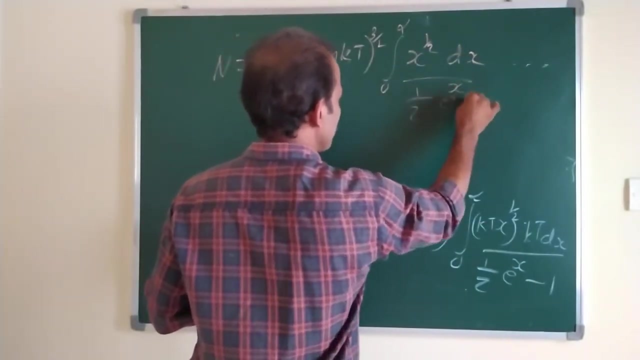 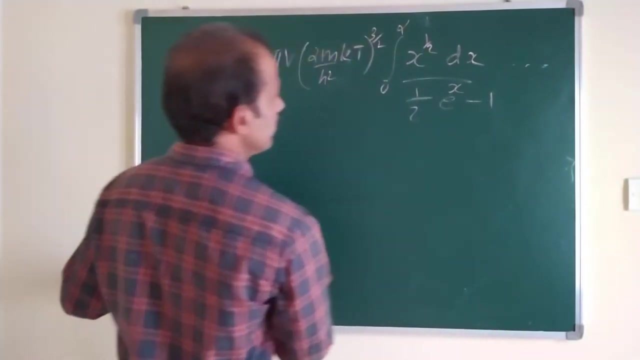 2m kt by s square kt is also 3 by 2.. In 0 to infinity, x rise to half remains into dx, divided by 1 by z, into: e raise to x minus 1.. Okay, e raise to x minus 1.. 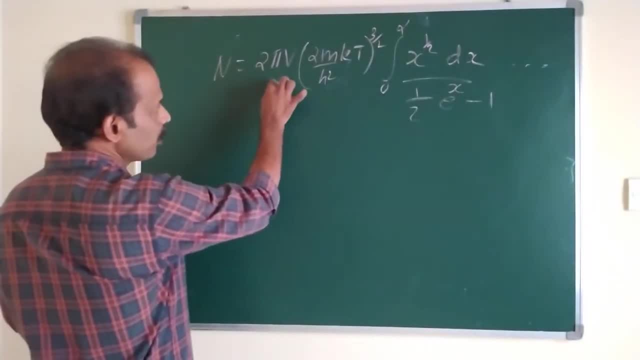 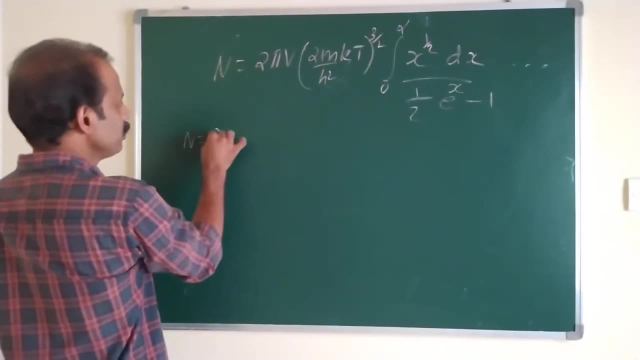 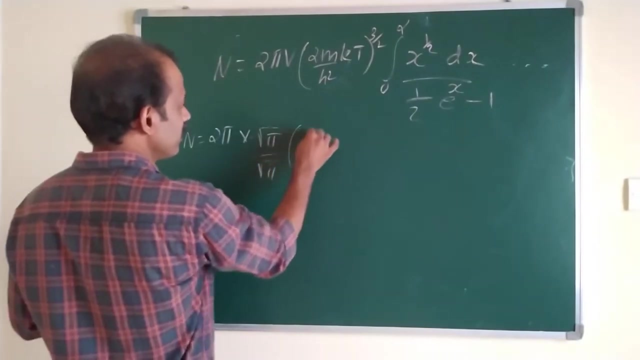 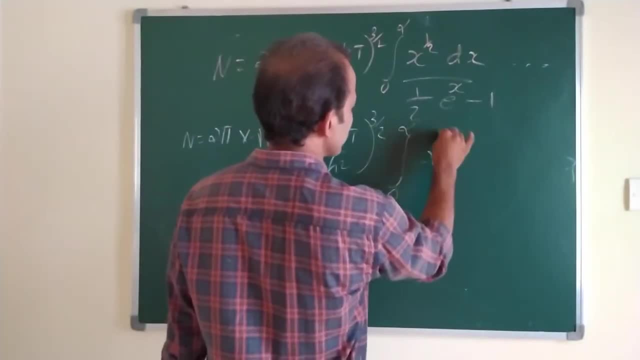 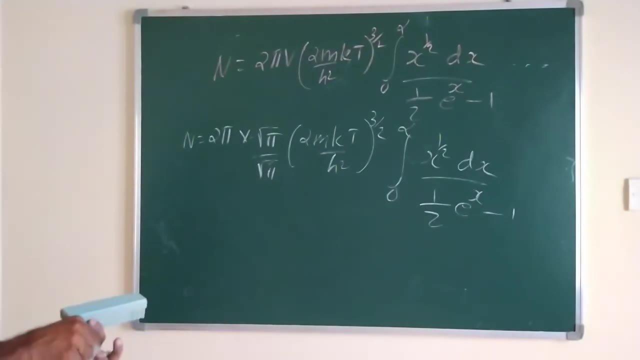 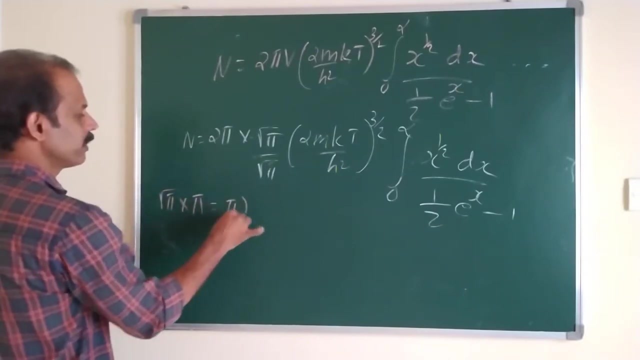 by 2, integral 0 to infinity. x rise to half dx divided by 1 by z into e rise to x minus 1.. But root pi into pi is equal to pi rise to 3 by 2.. So we can take it inside the bracket. 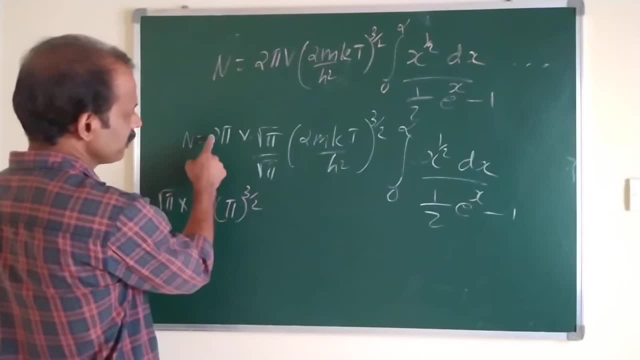 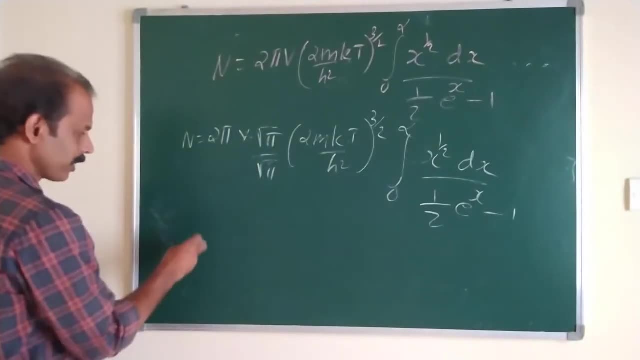 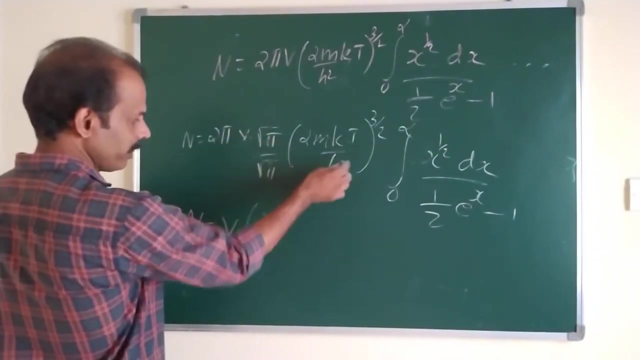 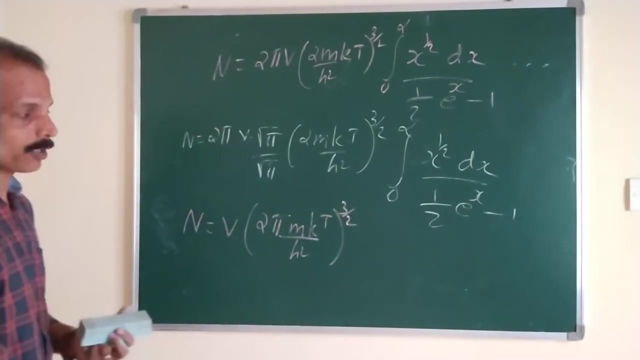 Okay, Remaining 2 by root pi into b, So this equation becomes: n is equal to b is here into 2 pi m. This pi m is 2 pi m. This pi m is 2 pi m, And pi and root pi inside 2 pi m, kt by s square volt rise to 3 by 2.. So pi in root. 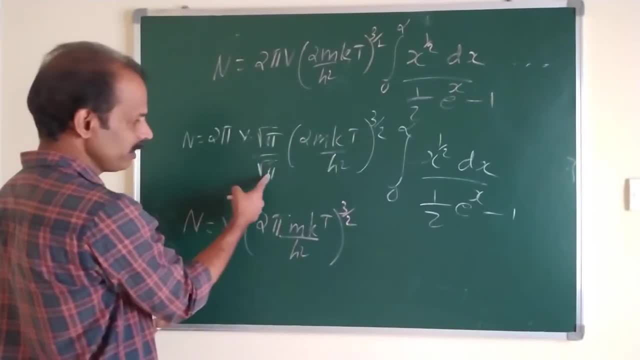 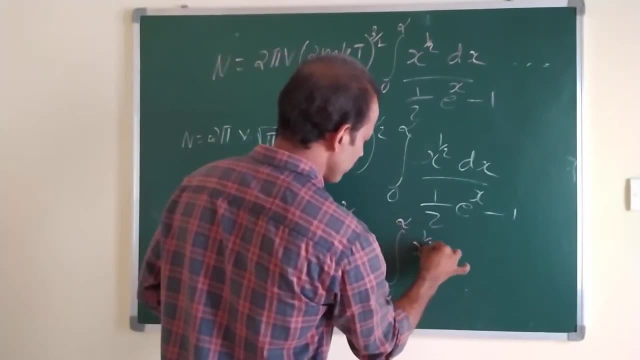 pi pi rise to 3 by 2 inside, and remaining 2 by root pi. 2 by root pi into integral. 0 to infinity. x rise to half into dx. divided by 1 by z into e, rise to x minus 1.. This term, 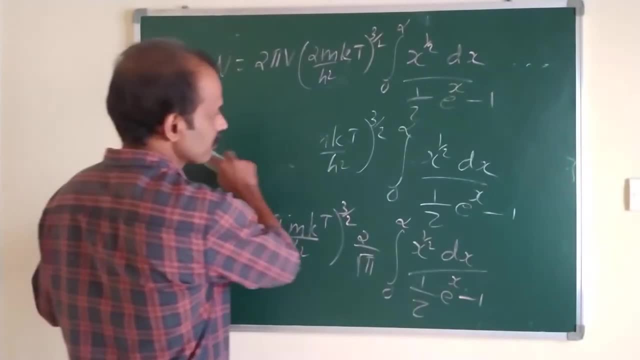 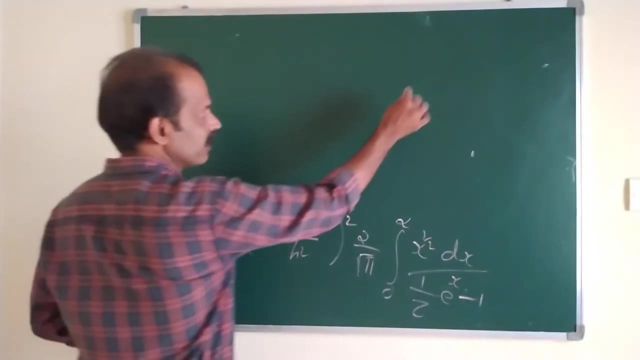 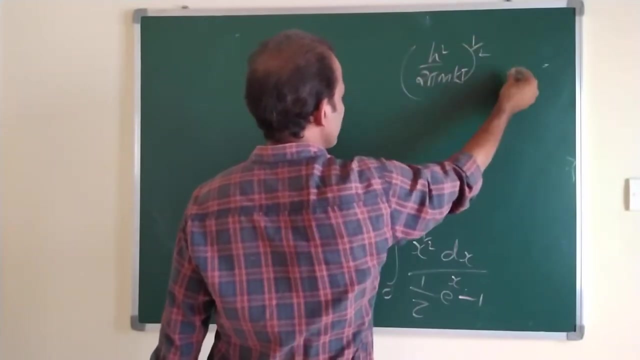 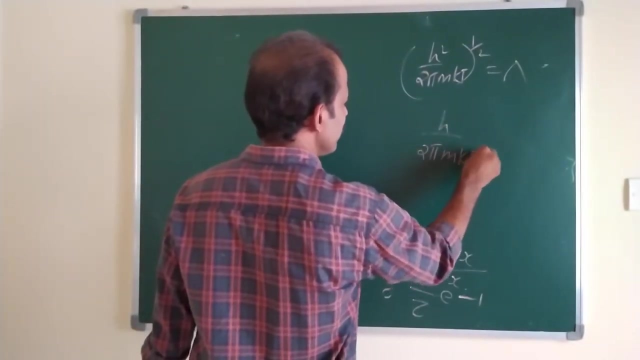 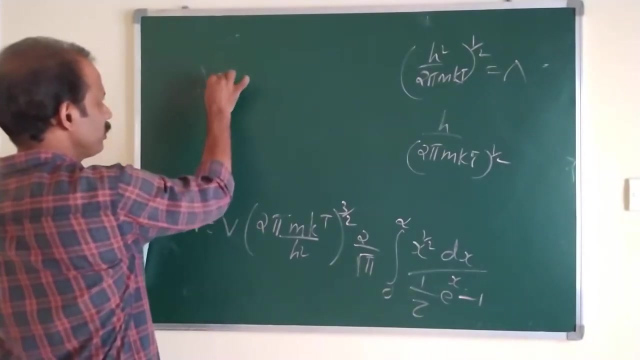 is very familiar, Very familiar, As we know. h by 2 pi m kt s square by 2 pi m kt volt rise to 1 by 2, is equal to lambda. Or h by 2 pi m kt volt rise to 1 by root- here You can write it like that, So nothing. 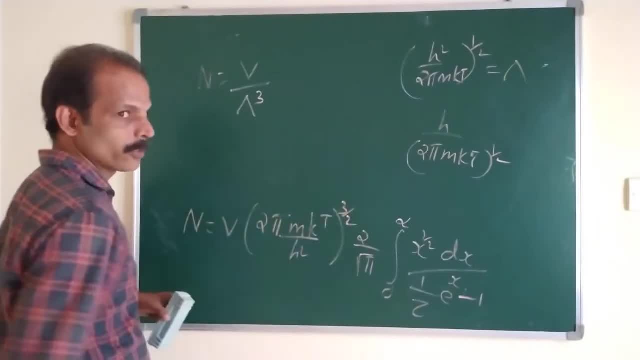 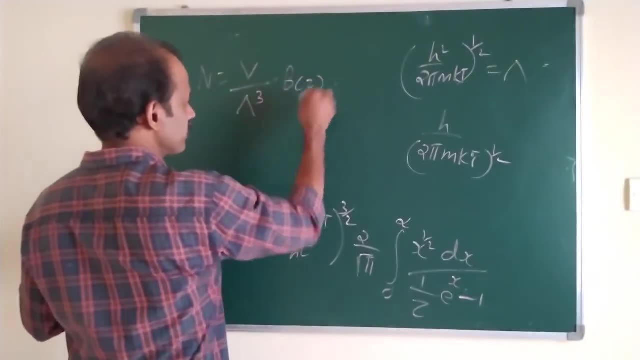 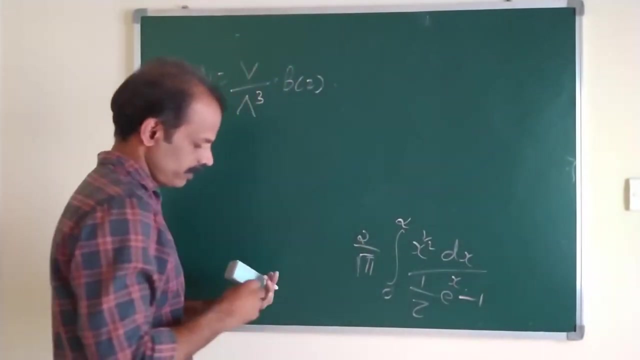 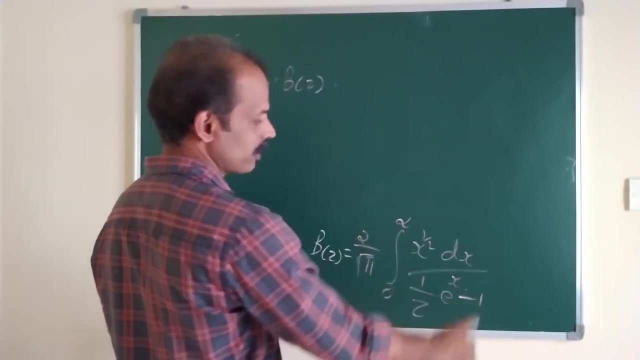 more. So h by 2 pi m kt v by lambda q, or you can write it as 2 pi m kt v by s square, or less 3 by 2, into b, where b z equal to 2 by root, pi integral 0 to infinity x rise. 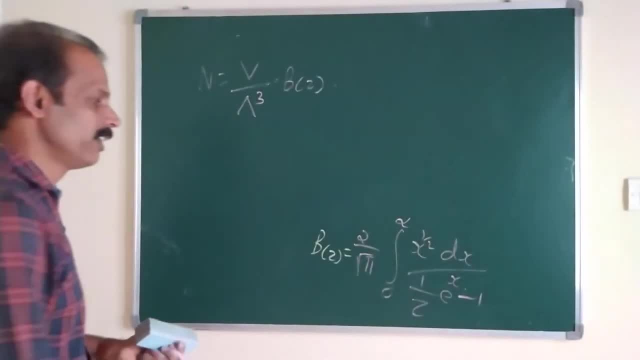 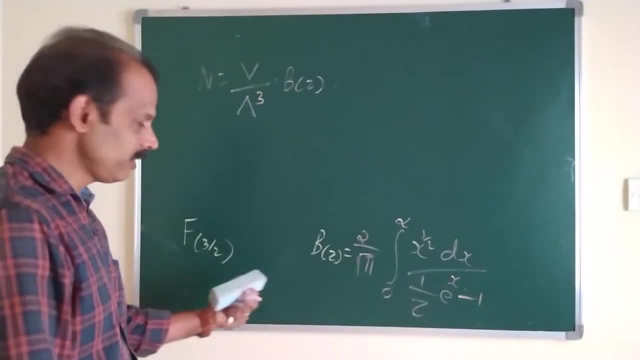 to half dx by 1 by z into e, rise to x minus 1.. In some cases we can write it like that. In some cases it is represented as f 3 by 2.. Instead of b of z, it is f of 3 by 2.. 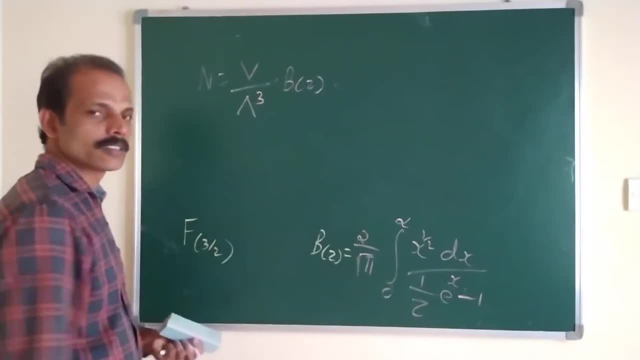 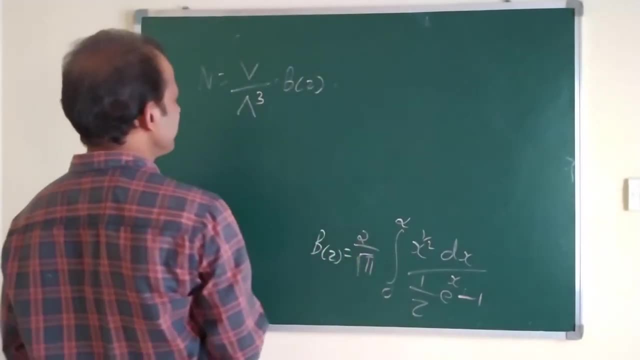 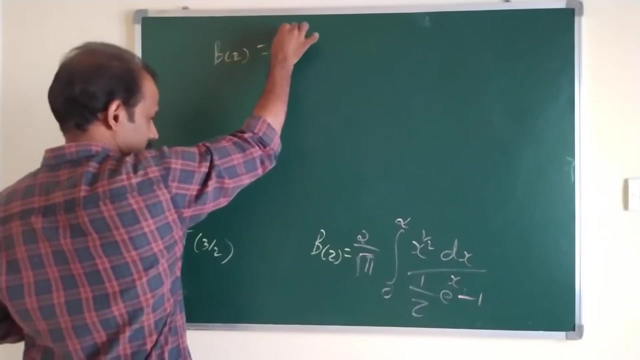 But similarly you can use either this one or this, It doesn't matter. So this one. So our equation is this: So b of z is equal to 2 by root, pi integral 0 to infinity x rise. 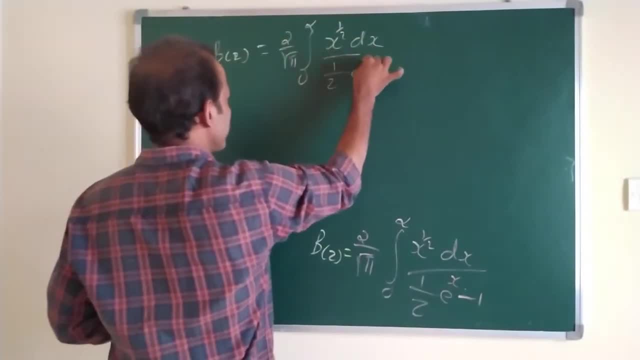 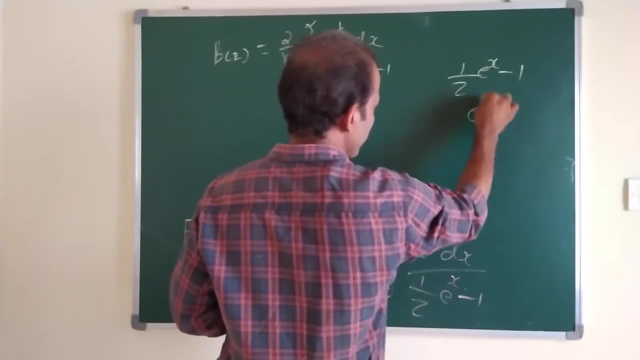 to half into dx. by 1 by z into e rise to x minus 1.. But this one, 1 by z into e rise to x minus 1, on cross multiplication we get z by z. So when we substitute here we: 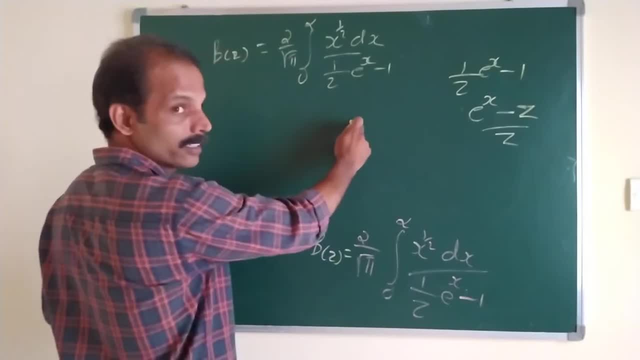 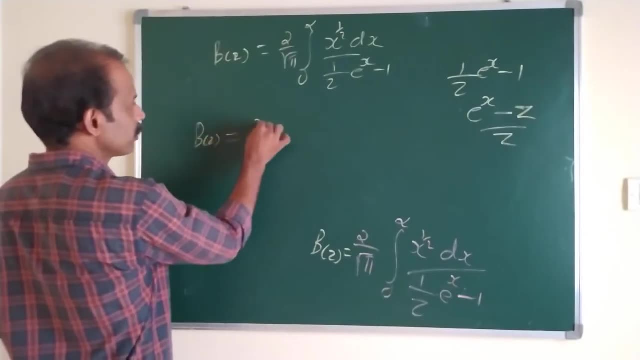 get e rise to x minus z by z. So this z comes to the numerator. So we get b. z is equal to root pi. root pi integral 0 to infinity x rise to x minus 1.. So this is the numerator. 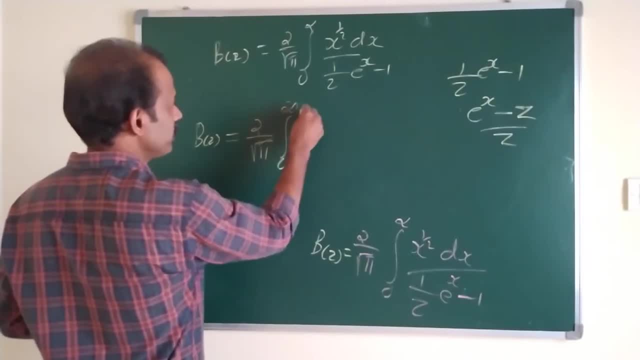 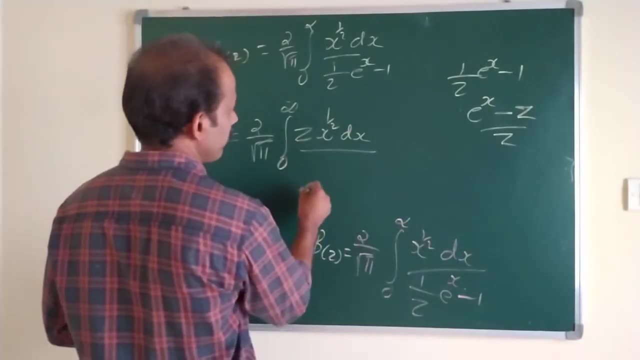 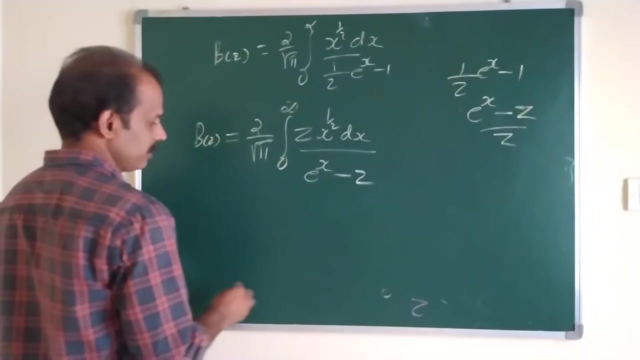 So we get b. z is equal to root pi, integral 0 to infinity. z into x. rise to half into dx by e rise to x minus z. But e rise to x minus z is equal to e rise to x into 1 minus. 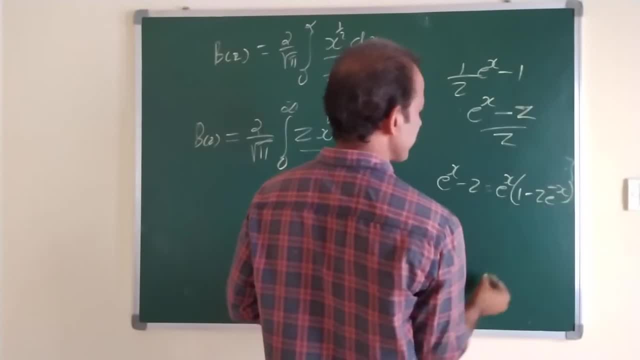 z into e rise to minus x. Okay, So e rise to x into 1, e rise to x minus 1.. So this is equal to 1, e rise to x. e rise to x into z. e rise to minus x, which is equal to z. 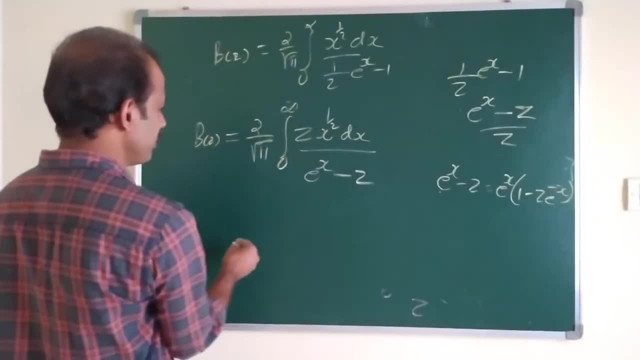 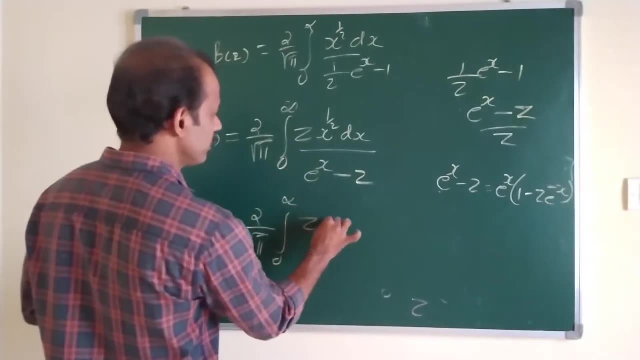 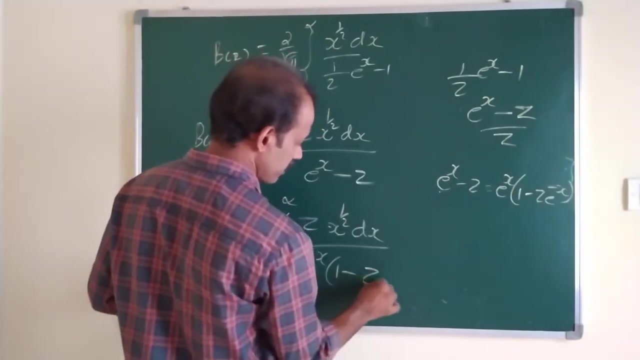 So instead of this we can write that equation: So 2 by root pi integral 0 to infinity. z into x. rise to 1 by 2 into dx by e: rise to x into 1 minus z. into e. rise to minus x. Take this: 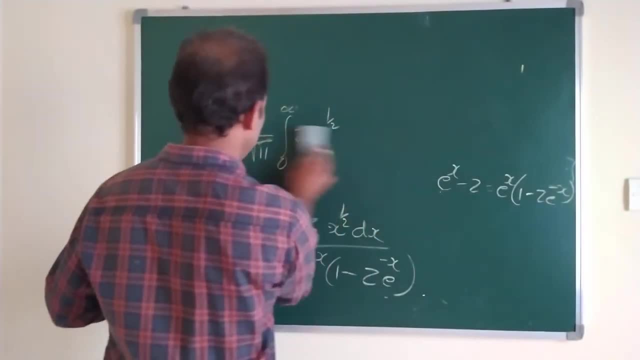 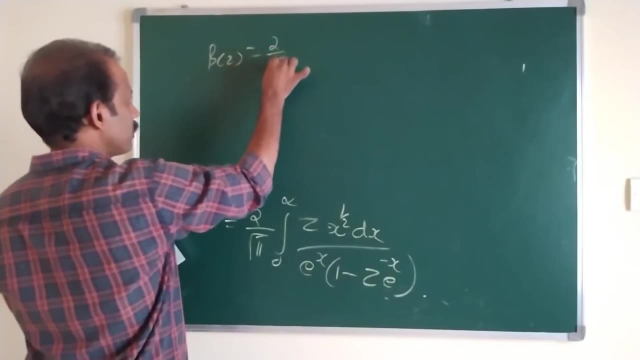 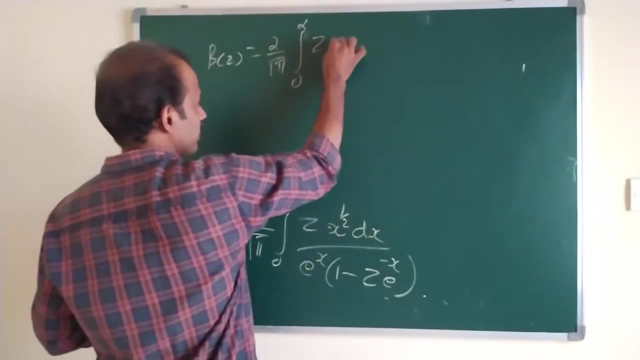 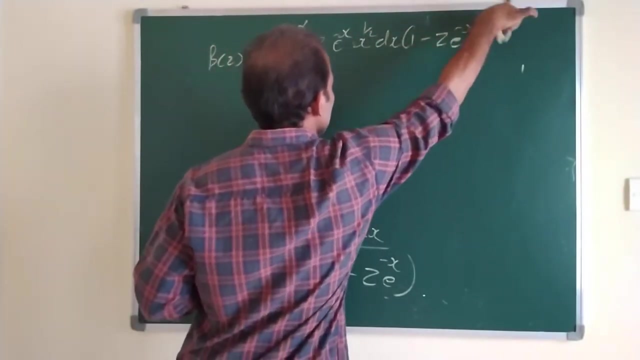 denominator to numerator. So we get b: z is equal to 2 by root pi integral 0 to infinity z e rise to minus x into x, rise to 1 by 2, into dx, into 1 minus z e rise to minus x, all rise to minus 1.. And it comes. 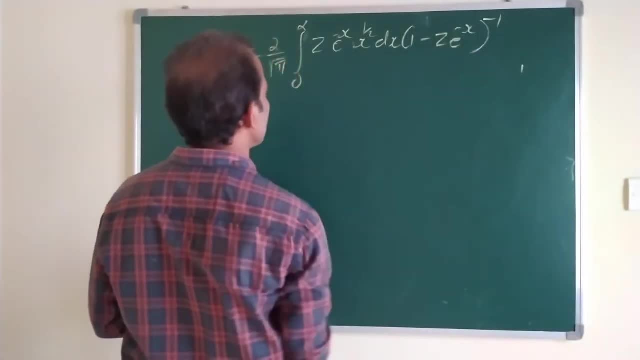 upside. So the integral of standard integral of this one expansion of that that is b, z is equal to 2 by root pi. integral 0 to infinity, z into x rise to 1 by 2 into dx, into 1 minus. 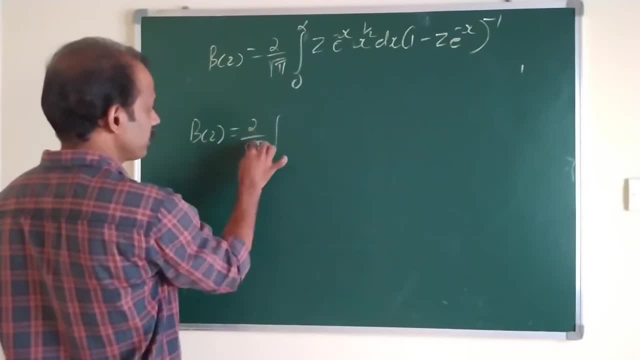 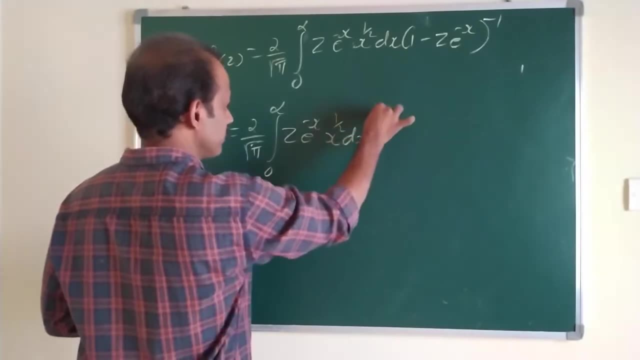 z e rise to minus 2 y z. This is equal to 2 by root pi integral 0 to infinity. z e rise to minus x. x rise to 1 by 2 into dx and 1 plus z e rise to minus x plus z. square e rise. 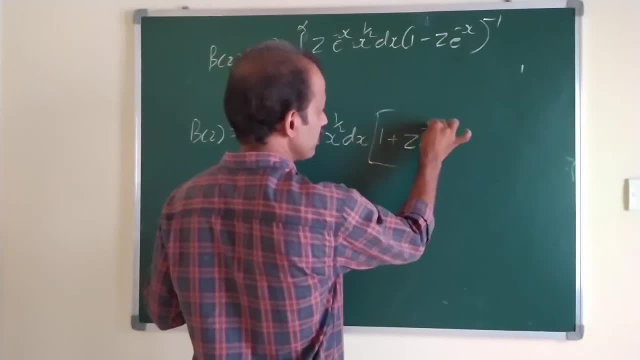 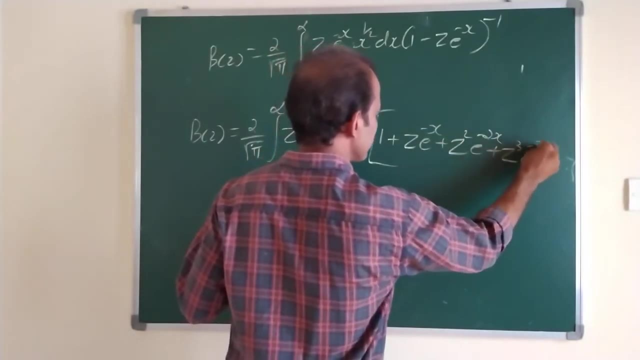 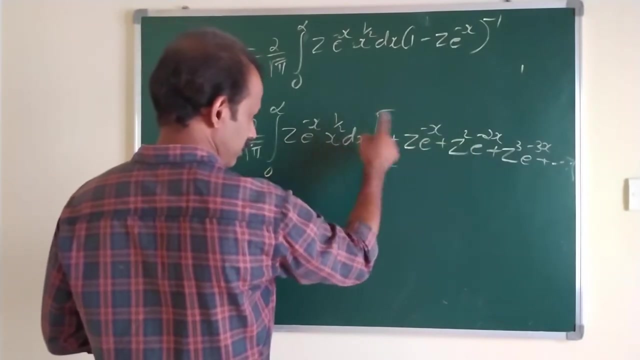 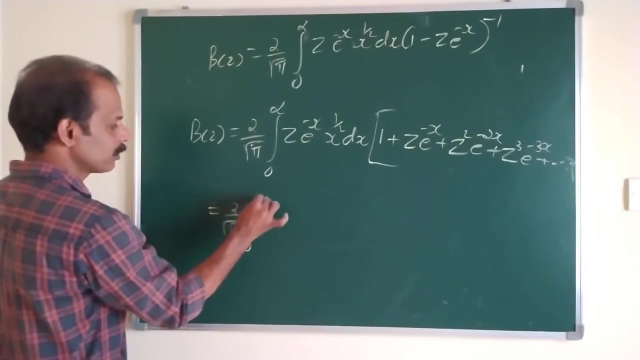 to minus 2x plus z, cube e. rise to minus x plus e. rise to minus 3x plus plus 3x plus d z. All right, Why this is arrestive? So this expansion, and on integration, we get 2 by root, 5, integral, 0 root 2, infinity z into. 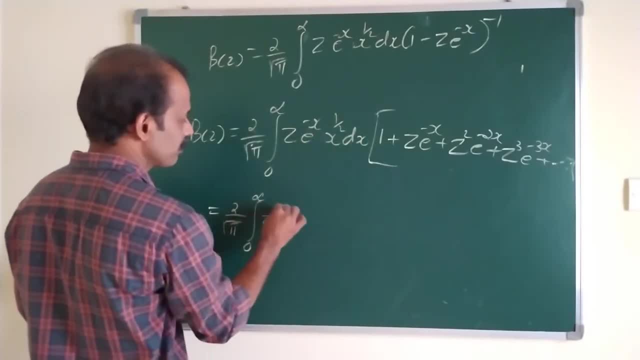 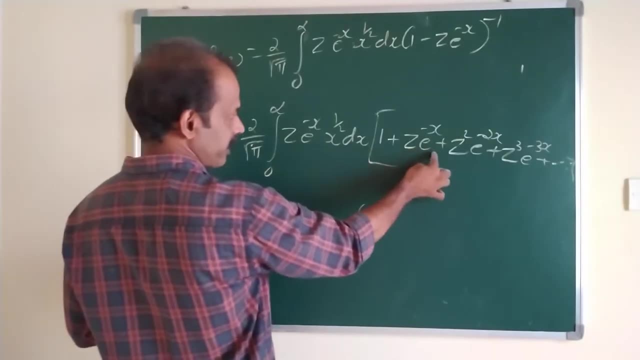 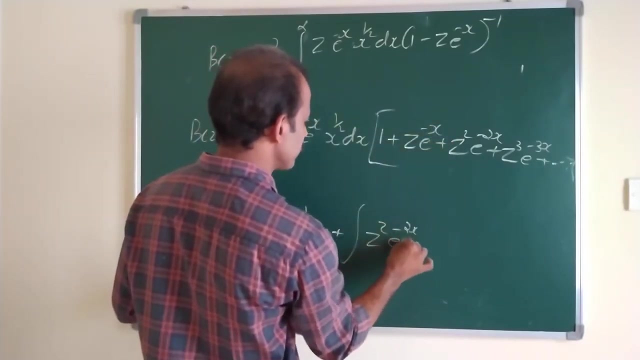 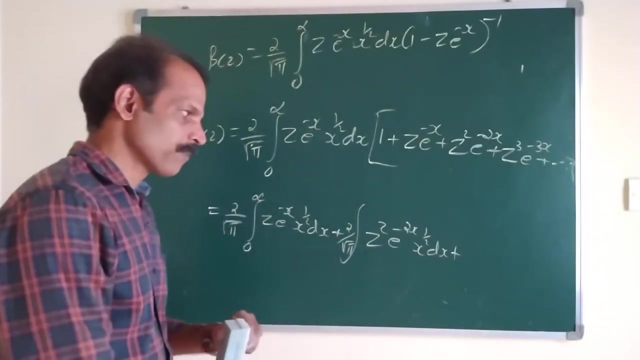 1 z. e raise to minus x into 1. e raise to minus x, x. raise to half into dx, the first term into 1, then the second term is this: that is z square. e raise to minus x, e raise to minus. e raise to minus 2 x. x. raise to half dx, sorry. e raise to root 2 pi, then 2 by root pi into integral. 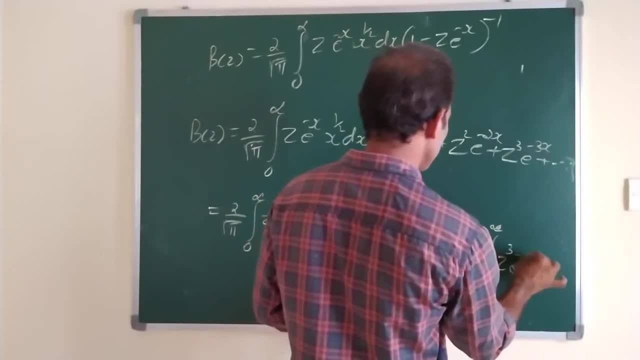 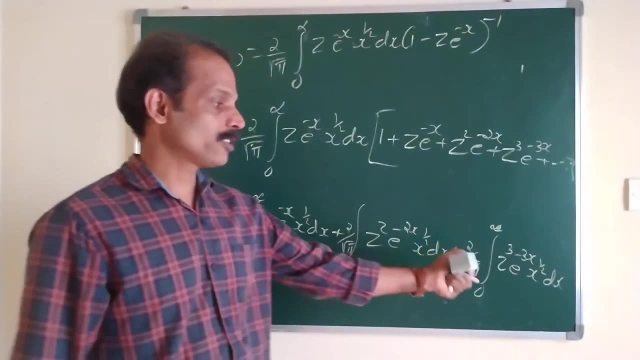 0 root 2. infinity. z cube. e raise to minus 3, x. x. raise to 1 by 2, dx. then z. raise to 4. e raise to minus 4 x. x. raise to 1 by 2, so on, and so on, and so on. 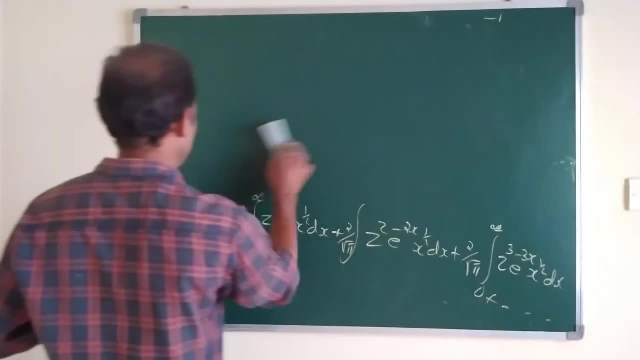 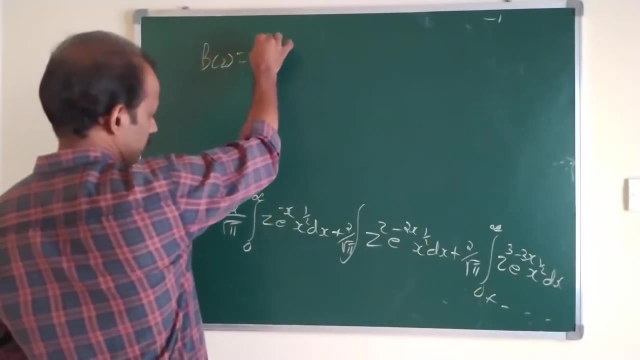 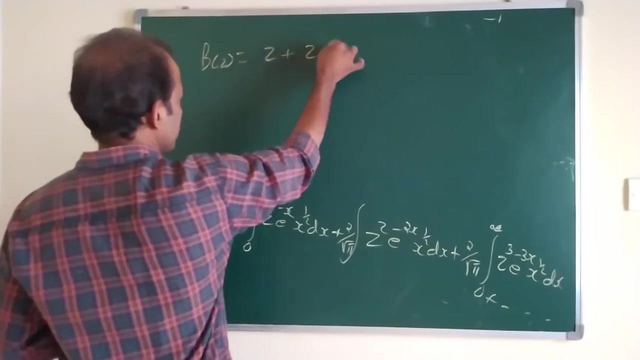 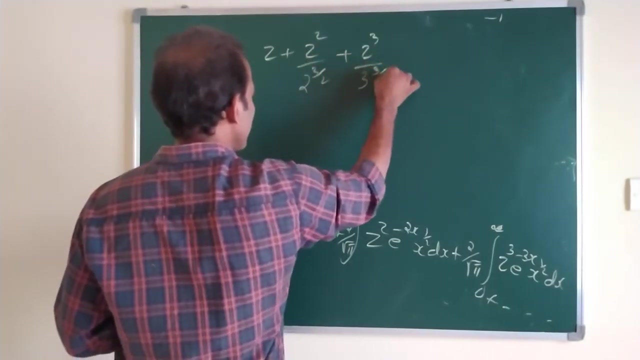 Thank you. The second integral of this is z plus z square by 2. raise to 3 by 2 plus z cube by 3. raise to 3 by 2 plus z raise to 4 by 4. raise to 3 by 2 plus z square by 2. raise to 3 by 2. 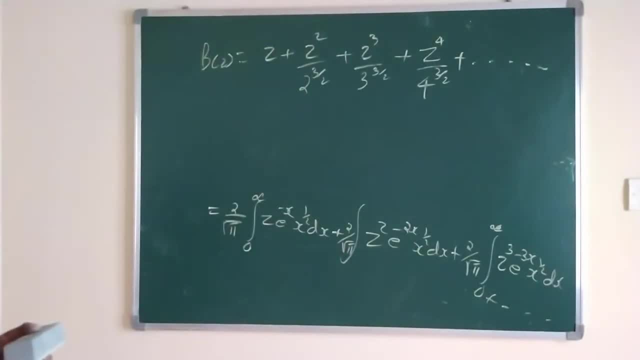 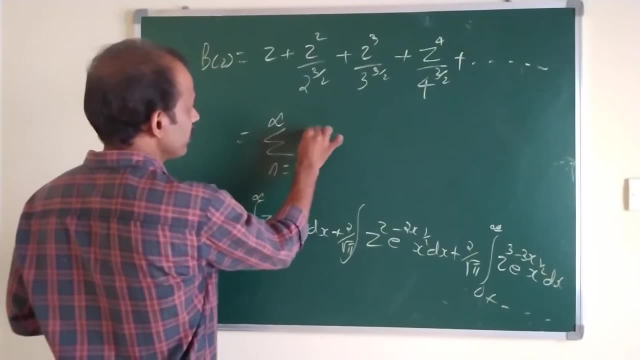 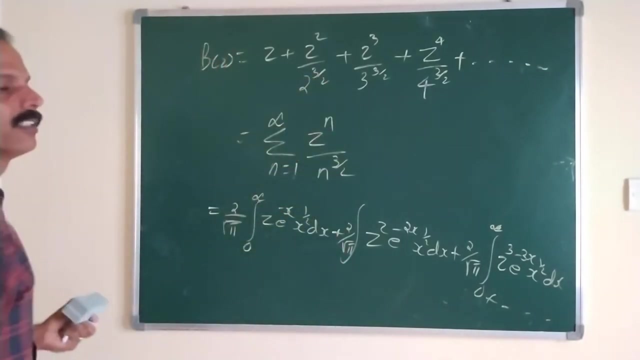 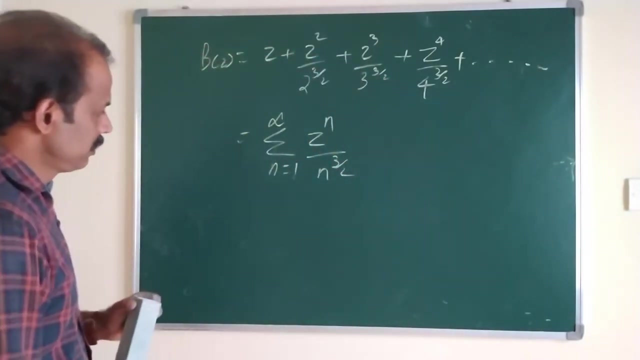 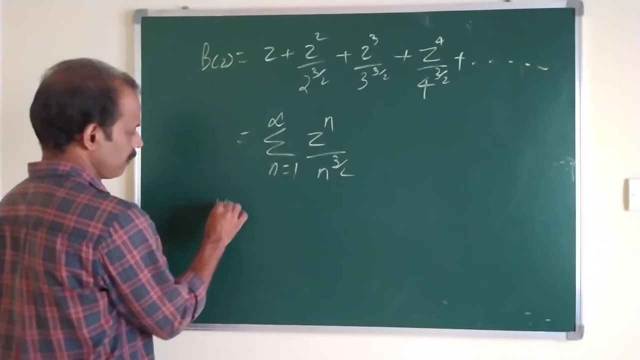 and so on. Now you can write this sigma: n is equal to 1 to infinity, z raise to n divided by n. raise to 3 by 2. that is the standard form of this summation. So at this point we need: and mu is equal to 0 or z is equal to 1. 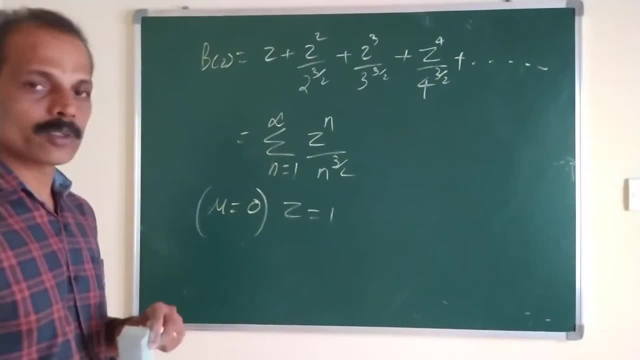 mu is equal to 0 or z is equal to 1, z is equal to e raise to minus beta mu, and mu is equal to 0 and e raise to 0, which is equal to 1. when z is equal to 1, this equation becomes: 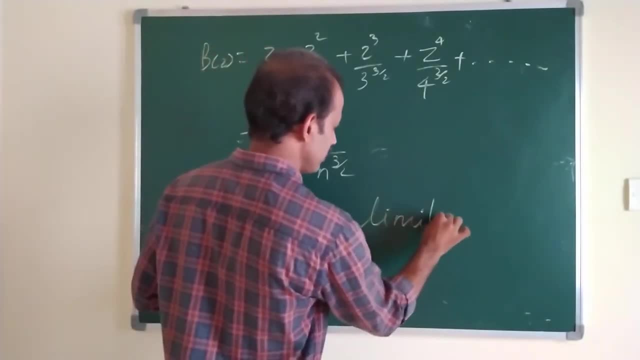 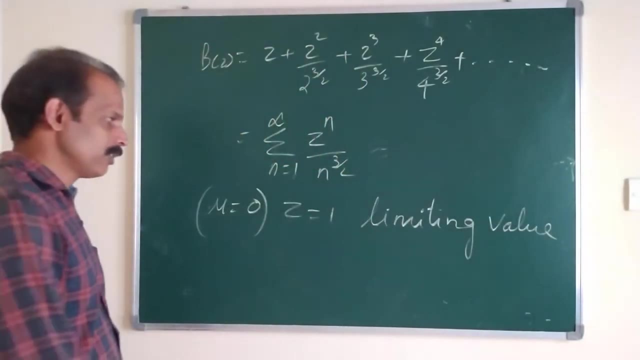 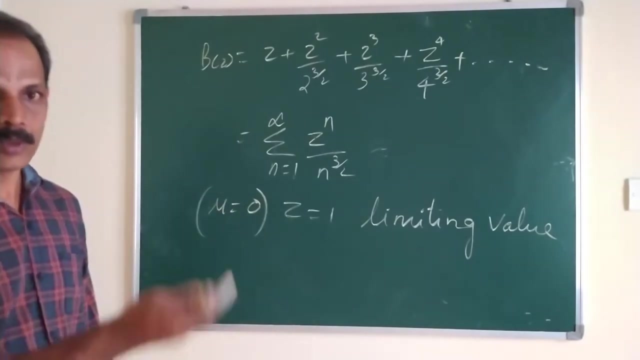 that is the limiting value. the maximum value of z is 1 and mu is equal to 0. you know the value of mu should be less than or equal to 0. the maximum value is 0. when it is 0, z is equal to 1. 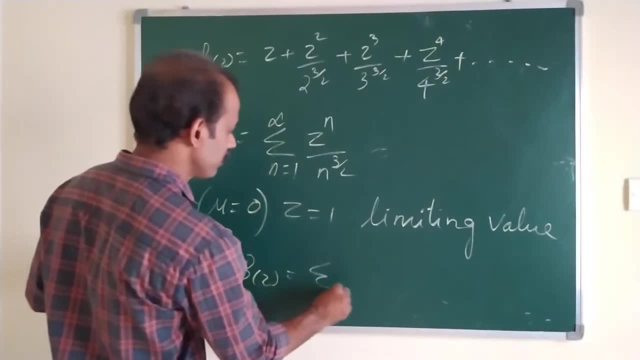 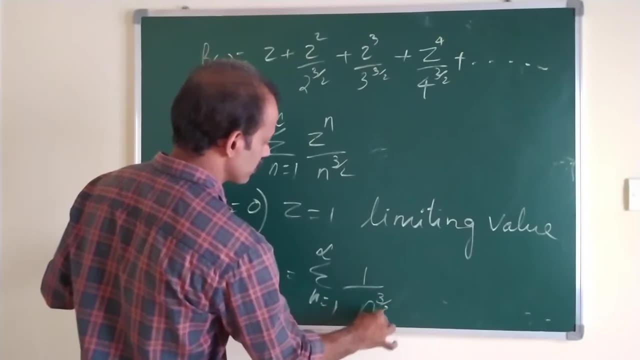 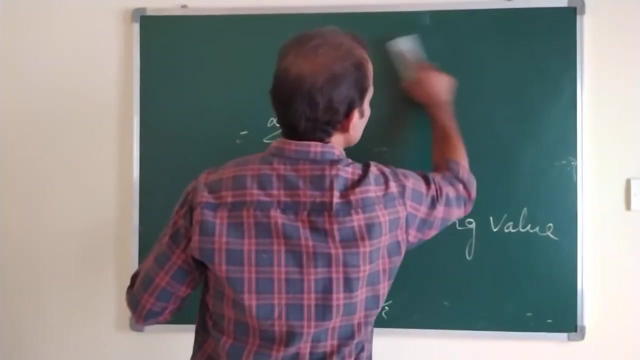 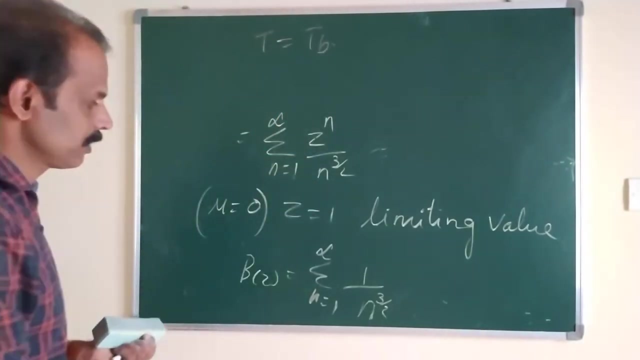 so this equation becomes: that is b of z is equal to sigma, n is equal to 1. to infinity, 1 divided by n raise to 2. when z is equal to 1, it is obtained at a temperature. it is obtained at a temperature. t is equal to t. 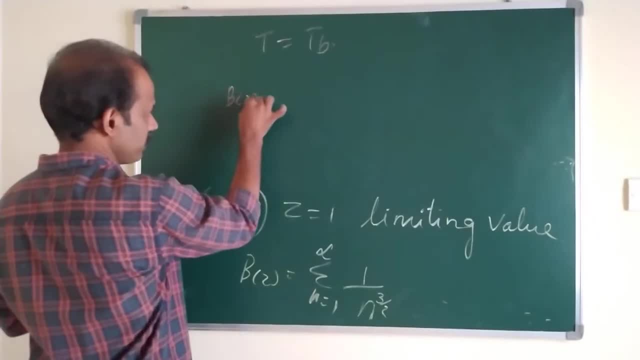 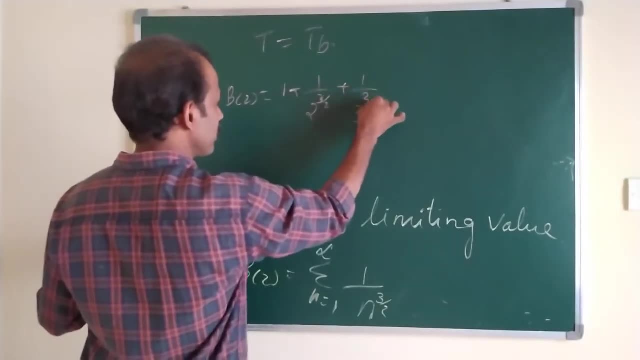 the expansion of this one that is b z is equal to expansion of this one is: 1 plus 1 by 2. raise to 3 by 2 plus 1 by 3. raise to 3 by 2 plus 1 by 4. raise to 3 by 2 plus plus, plus plus. 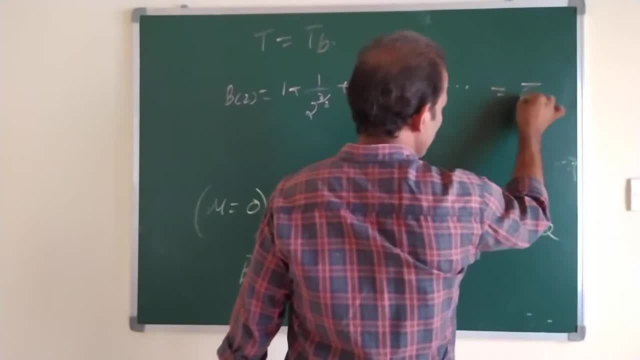 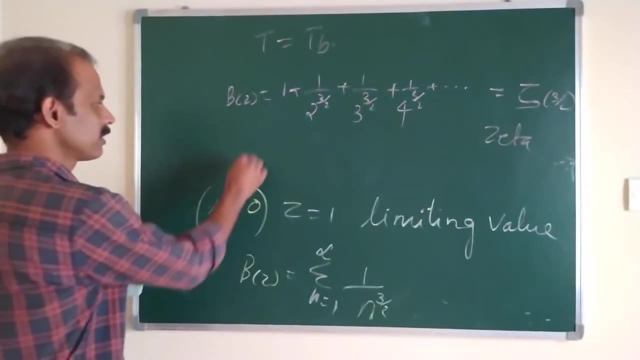 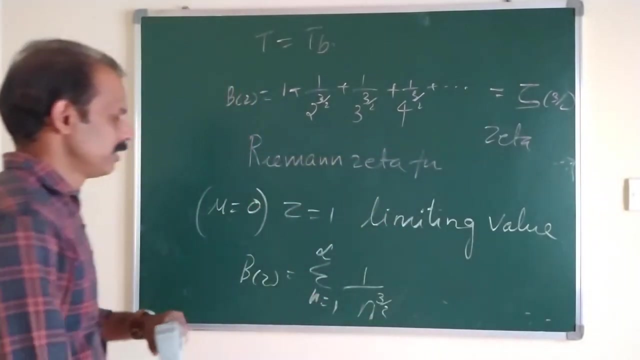 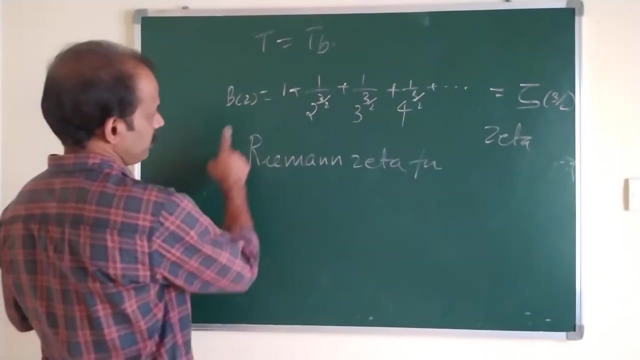 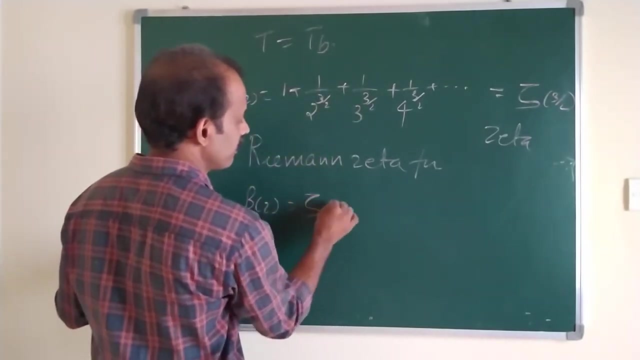 and which is equal to theta 3 by 2, the theta, it is known as a raymond theta function, and the value of which is calculate to this, which is equal to that is: b z. the value of this theta is equal to 2.612. 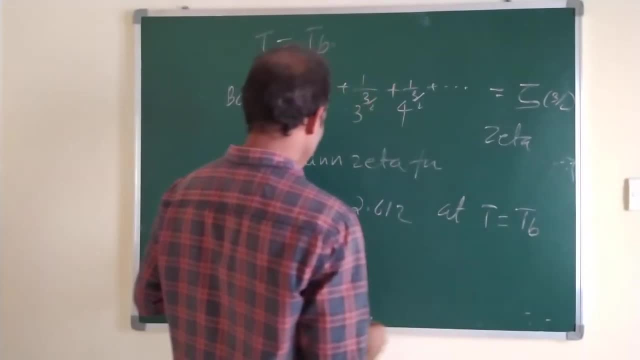 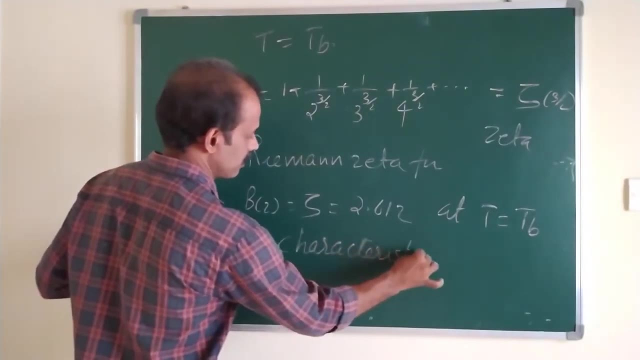 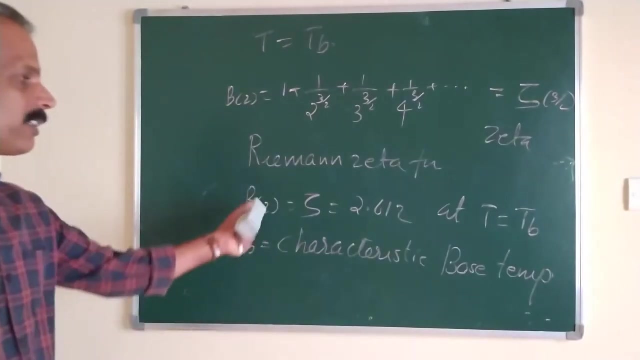 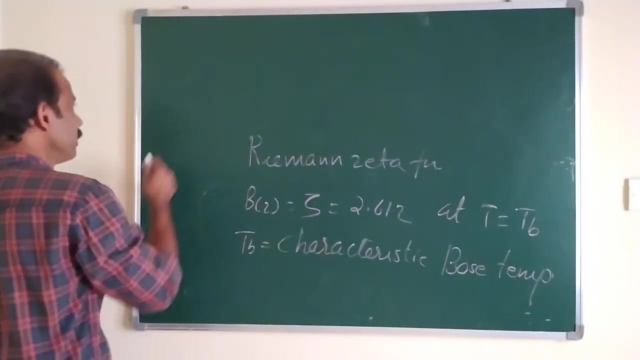 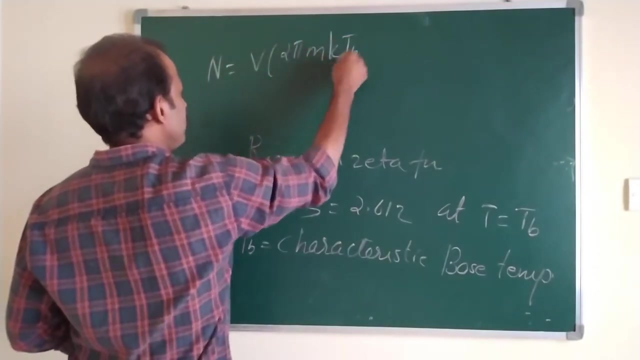 at temperature t is equal to t b. where t b is characteristic, both temperature. when temperature become t b, we get this value and on substitution of this b z value, we get the total number of particles. n is equal to v into 2 pi, m, k, t b. 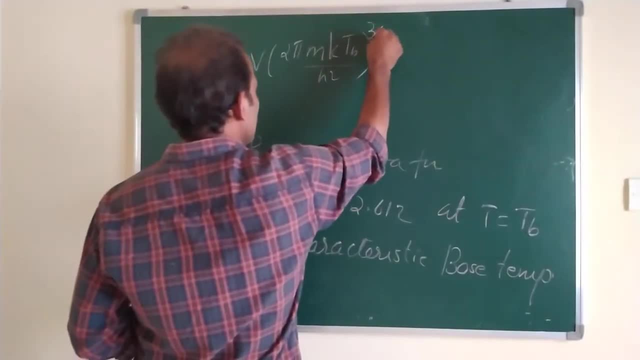 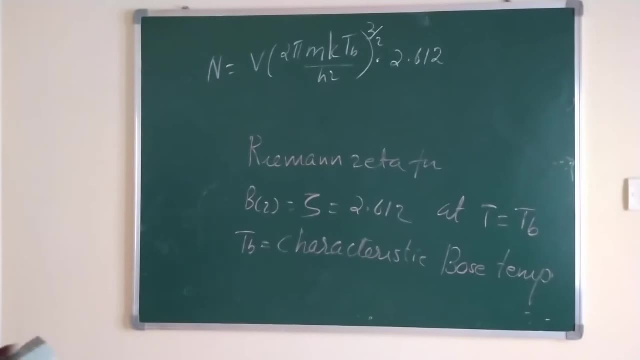 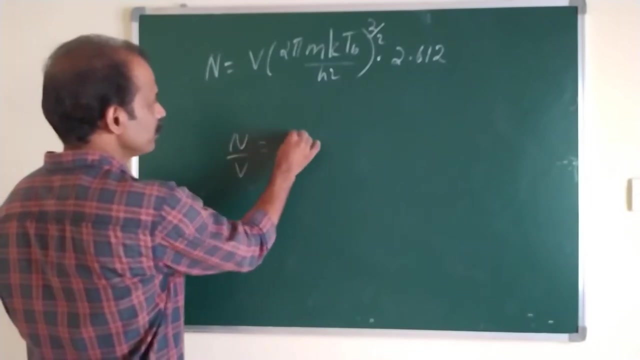 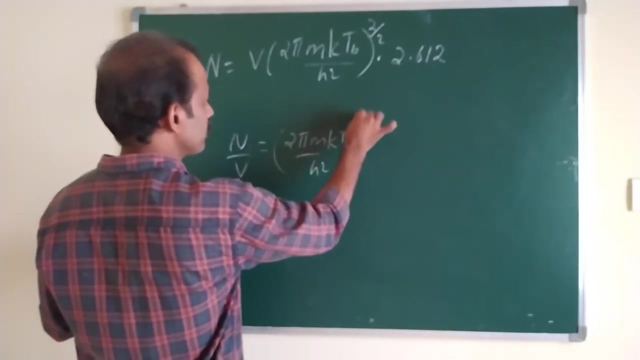 by x square all raise to 3 by 2 into 2.612 at t is equal to t b. now we can design t b as that is. t b n by v is equal to 2, pi, m, k. t by x square all raise to 3 by 2. 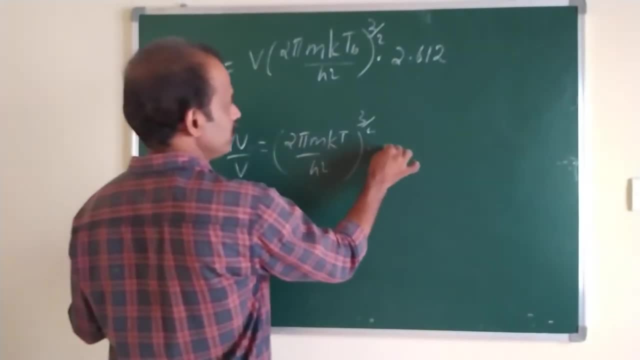 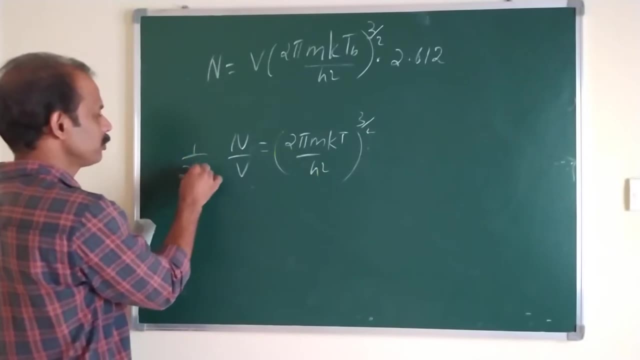 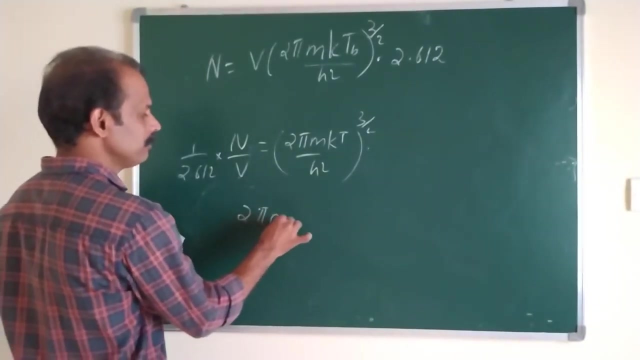 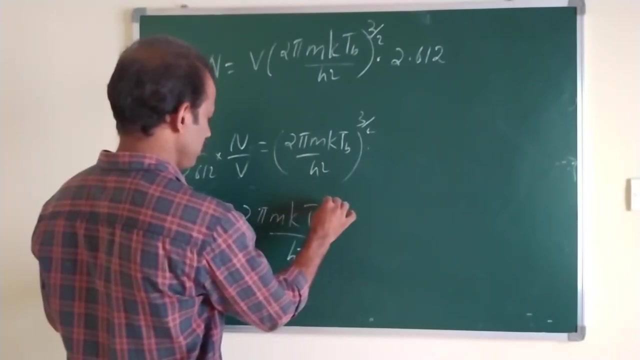 into 2.612. we can take this also this side, so we get 1 by 2.612 into n by v is equal to this much. or 2 pi m k t, sorry k t. b by x square is equal to n by v. 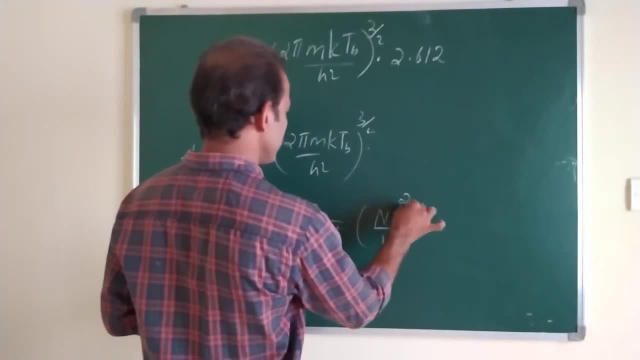 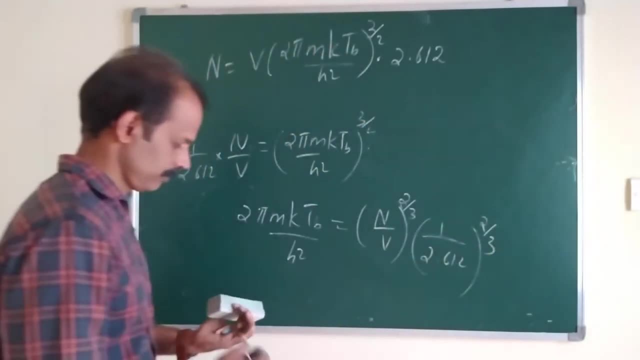 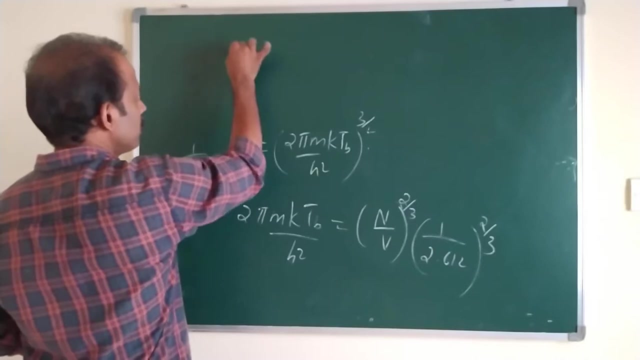 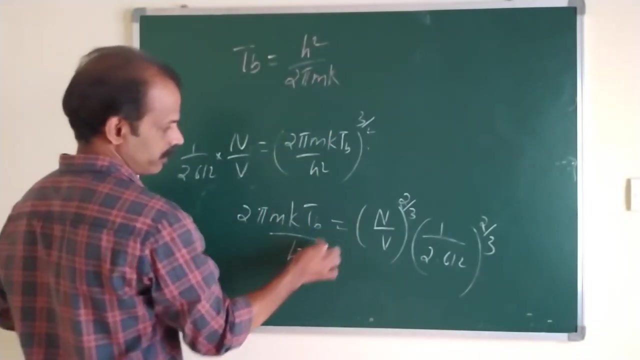 all raise to 2 by 3 into 1 by 2.612. all raise to 2 by 3, or t b is equal to x square by 2 pi m k, x square by 2, pi m k into n by v. all raise to: 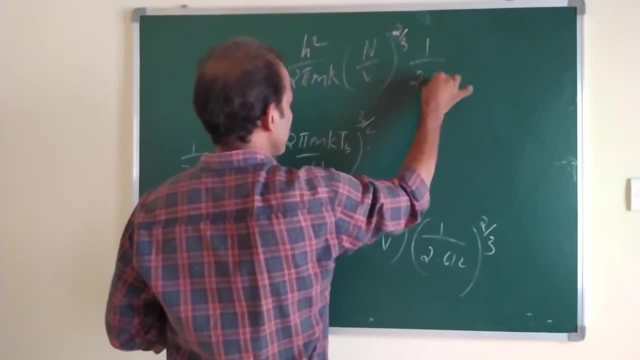 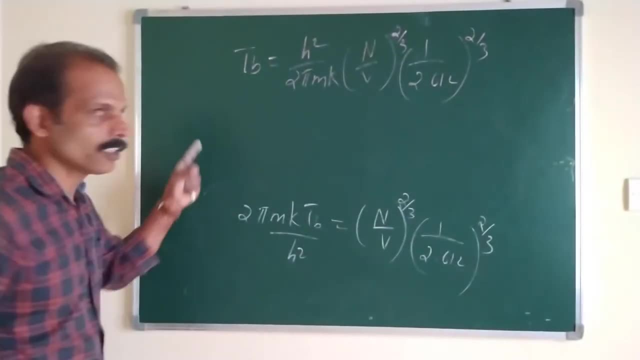 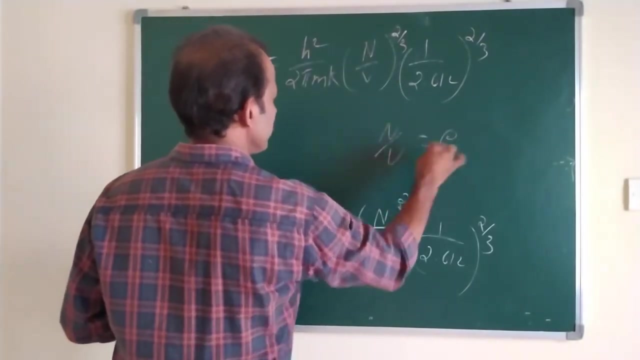 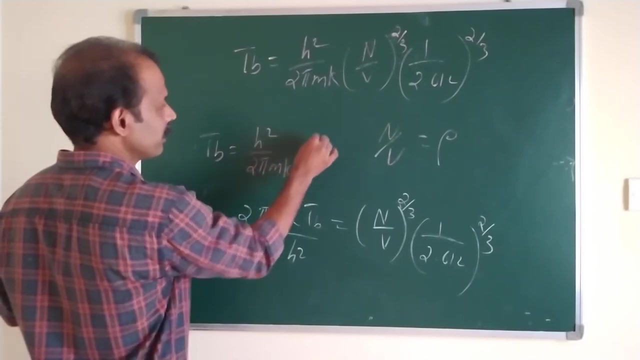 2 by 3 into 1 by 2.612, all raise to 2 by 3. that is the characteristic wasp temperature, which can be also written as: n by v is equal to density, so t b is equal to x square by 2 pi, m, k. 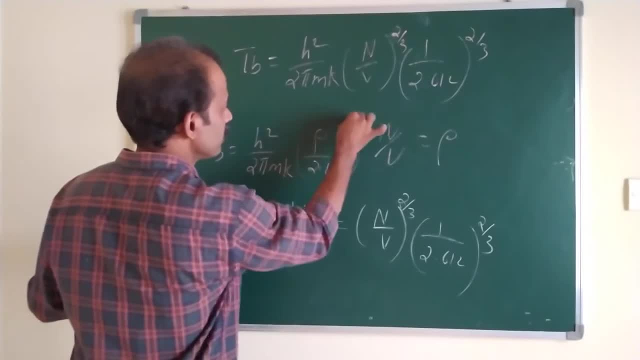 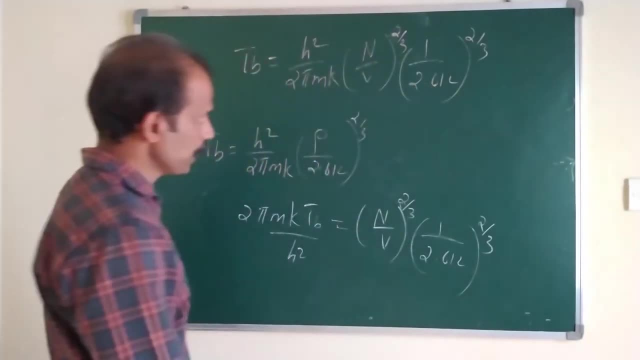 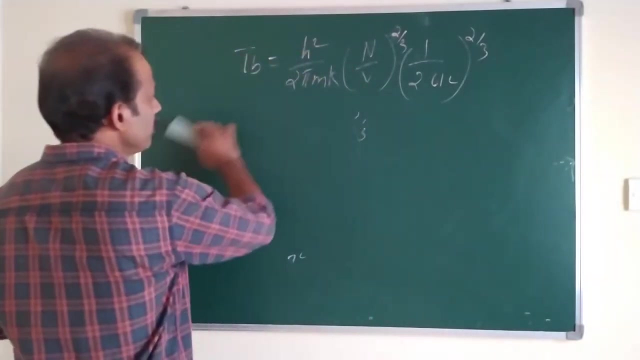 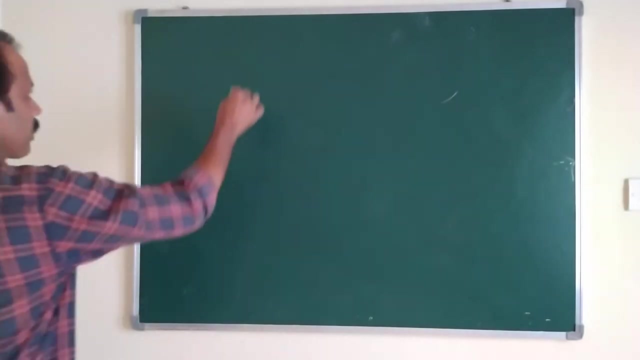 rho divided by 2.612, all raise to 2 by 3, can also represent like this: n by v is equal to rho. ok, so that is our characteristic boss temperature. then, moving back to our equation that is: at t is equal to at. t is equal to t b. 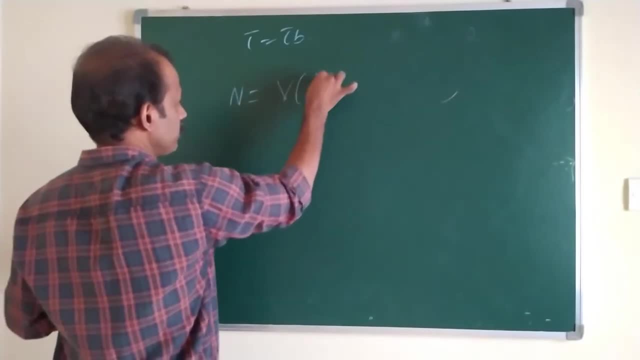 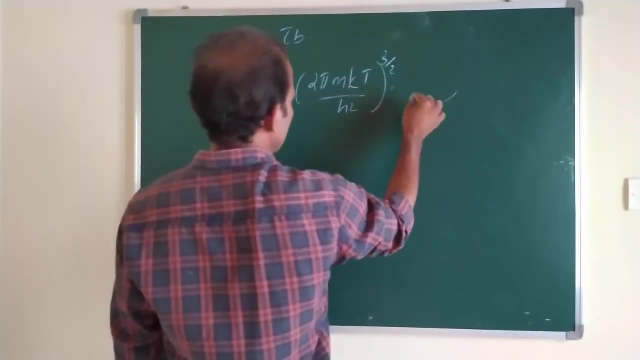 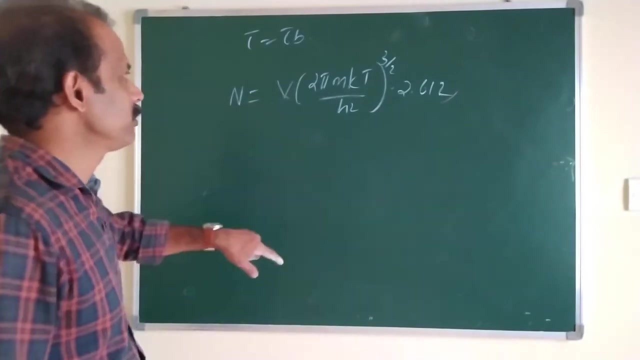 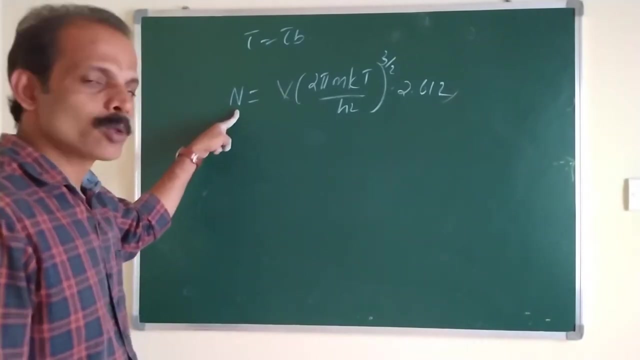 dot. number of particles is equal to v into 2, pi, m, k, t by square, 3 by 2 into 2.612. that is our equation. suppose temperature is decreasing this t b. actually, suppose it is decreasing what will happen? the number of particles also. 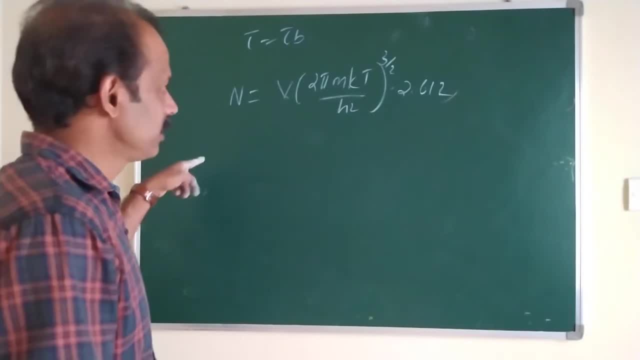 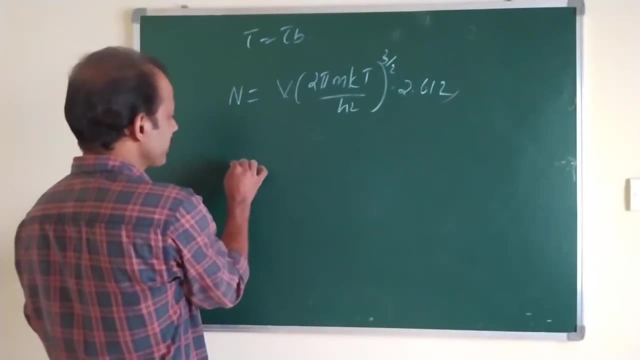 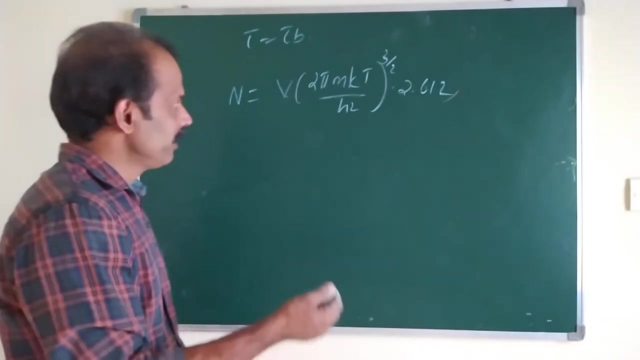 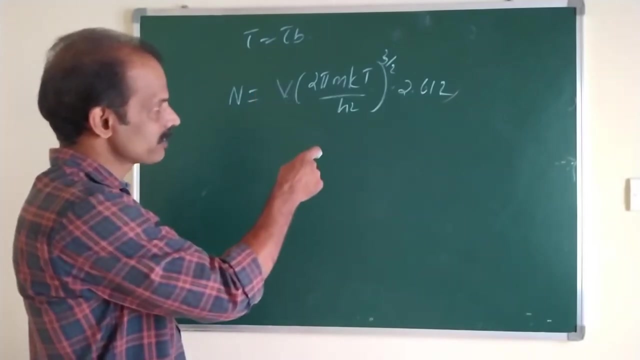 decreases. right. as the temperature is decreasing, number of particles also decreases. actually, at lower temperature the particles get down to ground state. that is, ground state is more and more populated and as the temperature increases, the excited state gets populated here, as the temperature decreases, number of particles decrease. 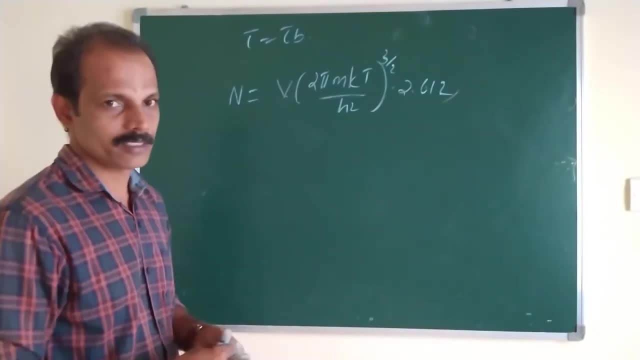 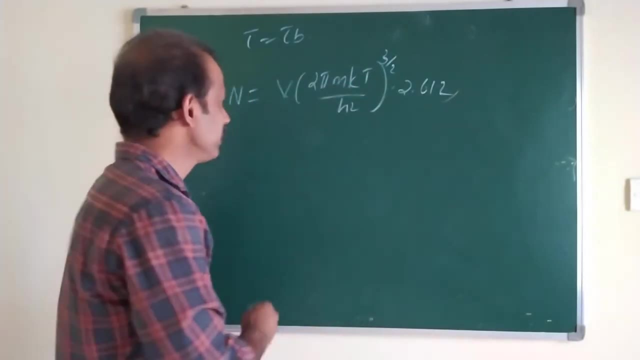 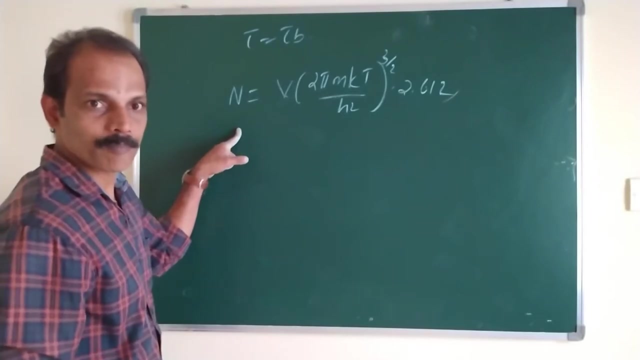 that is, total number of particles decreases. how it is possible? it is not possible. total n is total number of particles. total number of particles never change with temperature, but n by v change with the temperature. total number of particles per unit volume. number of particles per unit volume may. 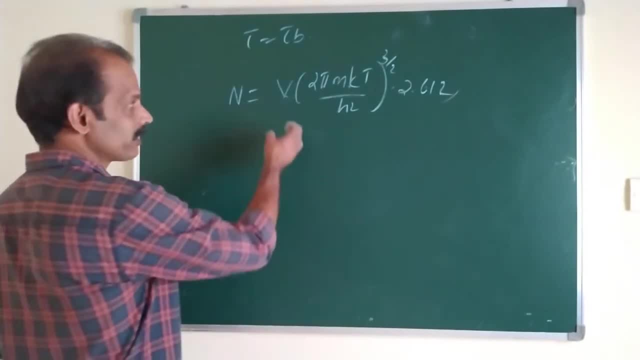 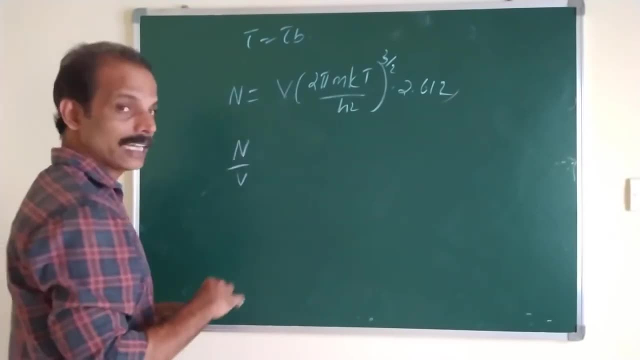 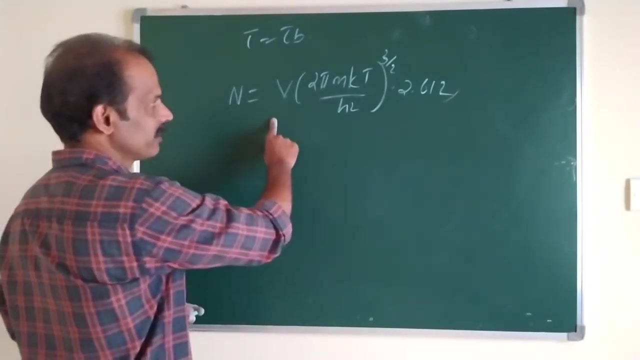 change that depends upon temperature. as the temperature varies, volume also changes. so n by v can change, but n never changes as temperature decreases or increases. but according to this equation, according to this, all these are constants. suppose v is constant, t, pi, m, k, h, all are constants. 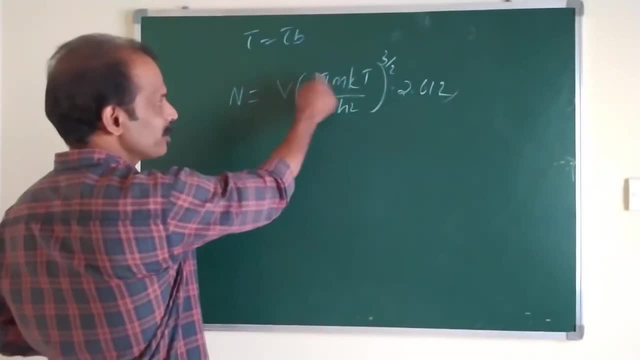 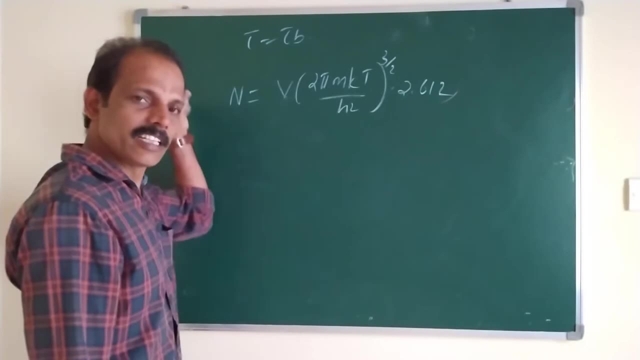 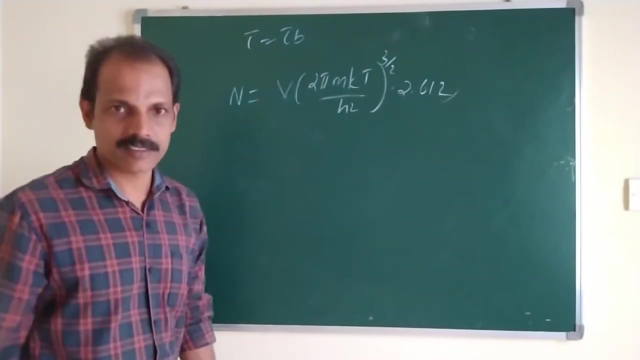 this also equals to a constant value. this also a constant value. then n is proportional to 3 by 2, right. as temperature increases, number of particles increases. as temperature decreases, total number of particles decreases. so something went wrong when we are deriving this equation. something happened, the equation is not satisfied. 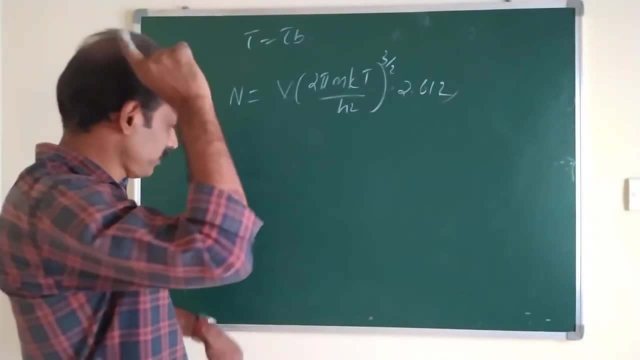 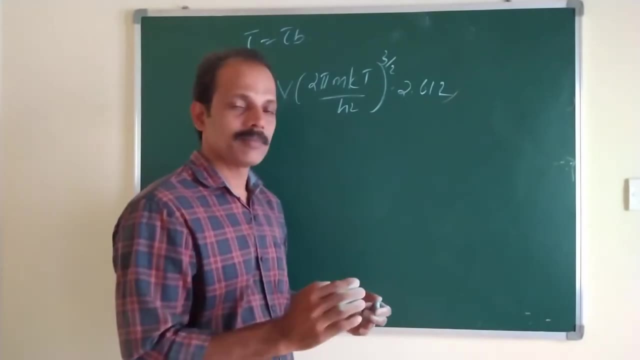 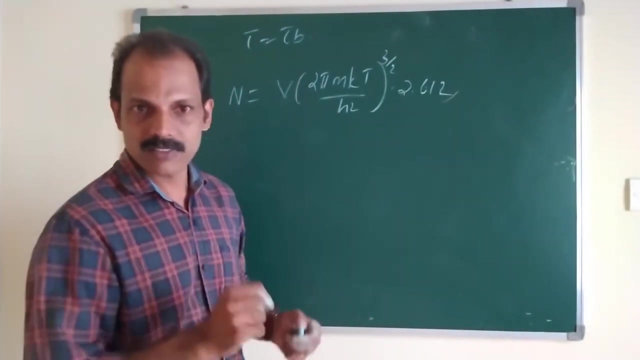 right, that is the first term. I told you that the first term of the summation, that is ground state g i by e raised to beta, into e minus mu minus 1, when v is equal to 0 and in the ground state e 0 is equal to. 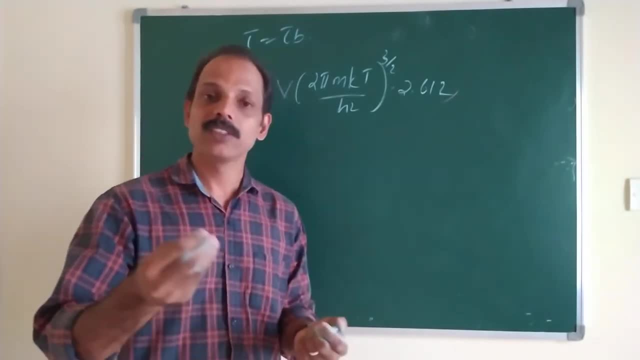 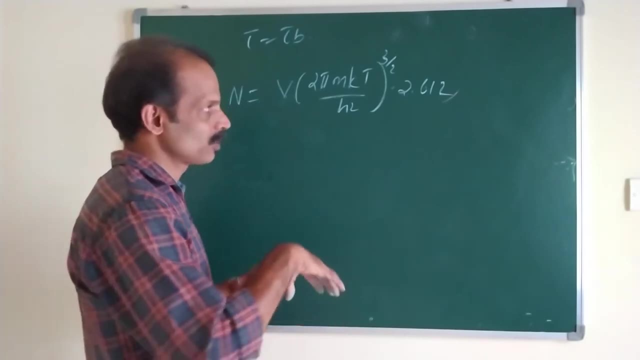 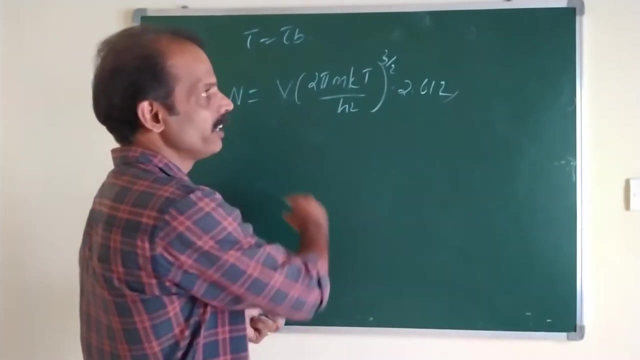 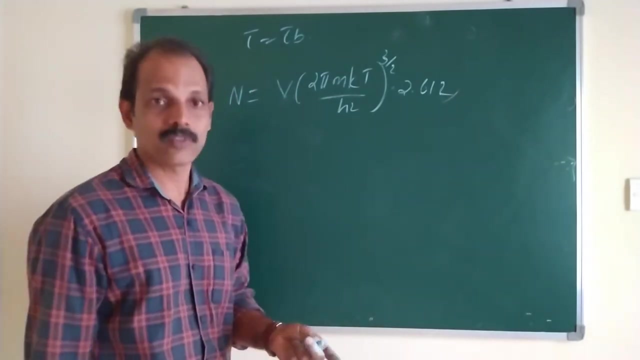 e is equal to 0. then e raised to b, beta term becomes 0. that so that all term vanishes. so we are omitting that term and converted to integration. that omission affected us, so integration effect seriously makes some error in this derivation. so we have to. 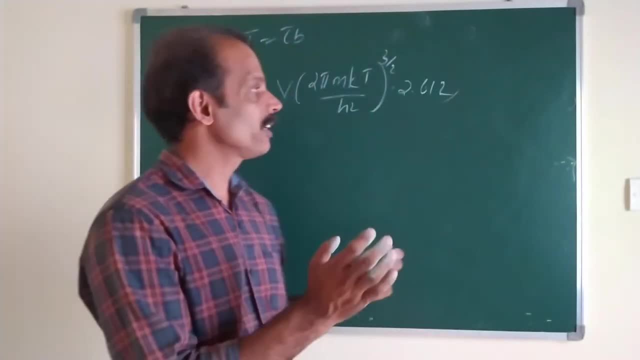 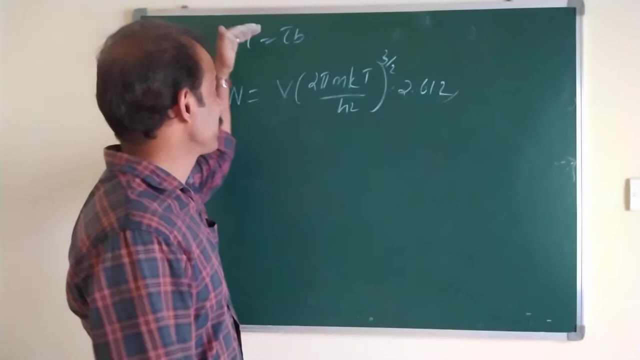 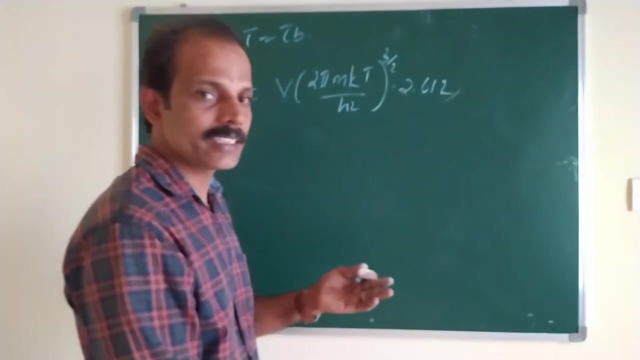 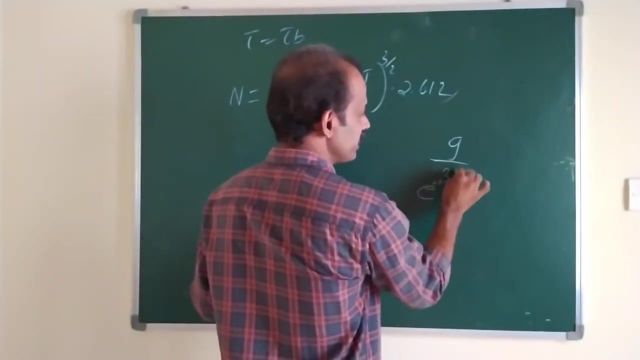 consider the ground state level. ground state level of the system bosons. ground state level of the gas, also at lower temperature, as the temperature decreases at lower temperature, ok, so at lower temperature. we are also including the ground state term. ground state term is g i into beta. 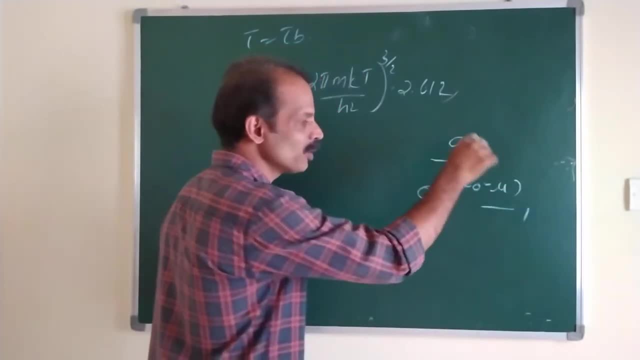 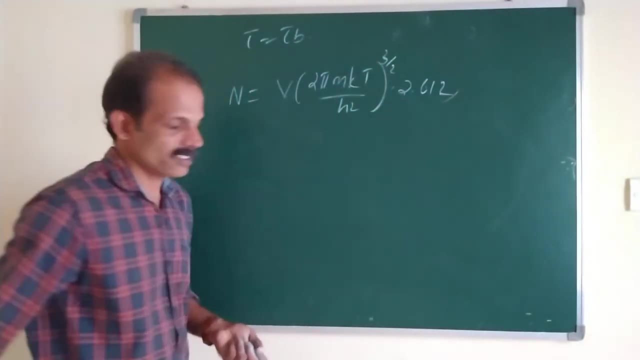 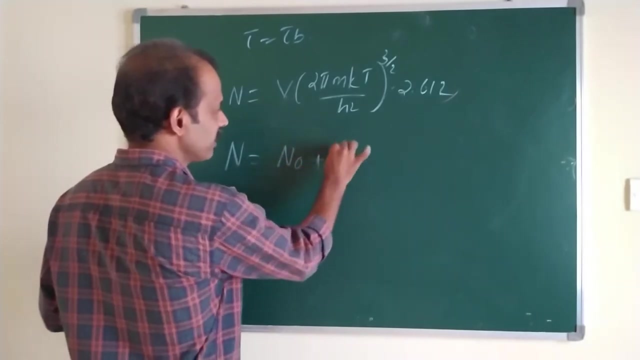 e, 0 minus mu minus 1. this term also we are including, so we have the total number of particles then should be equal to: total number of particles should be equal to n 0 plus n e, where n 0 is the number of particles present in the ground state. 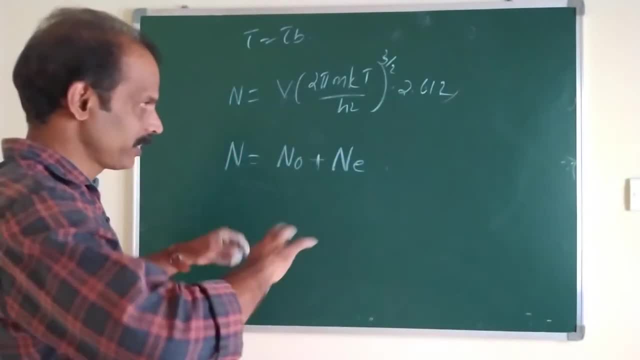 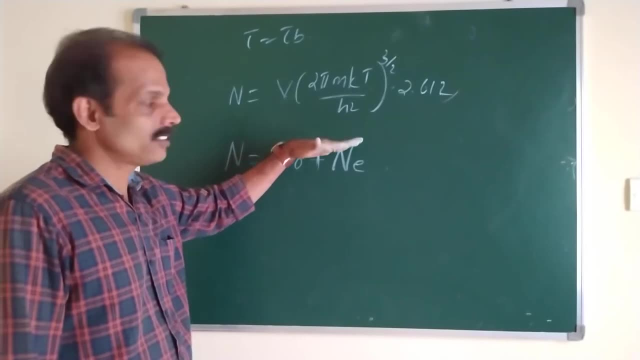 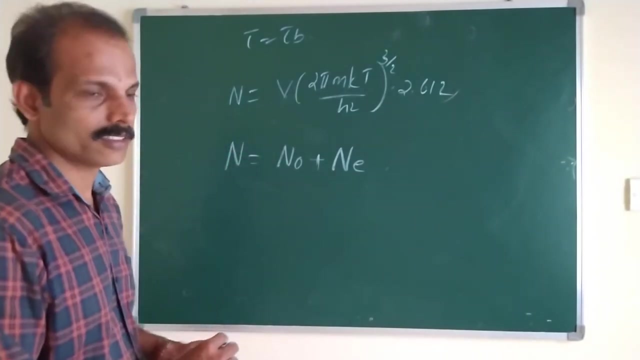 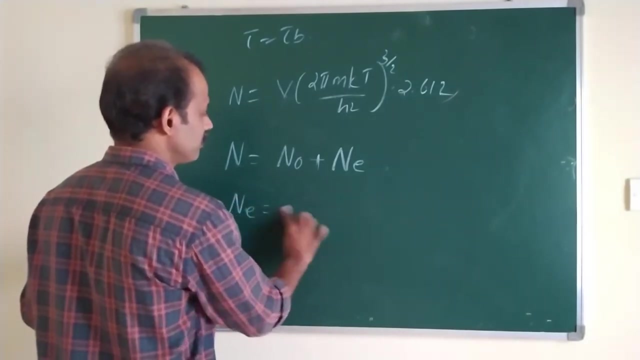 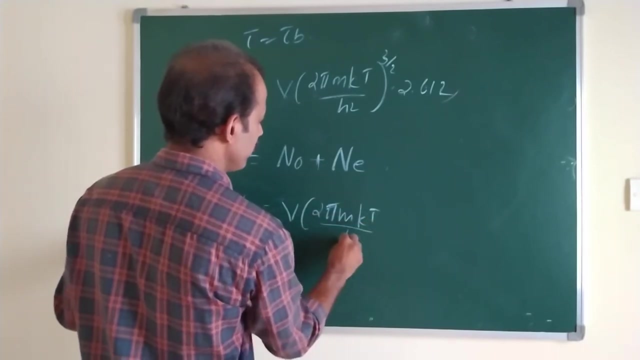 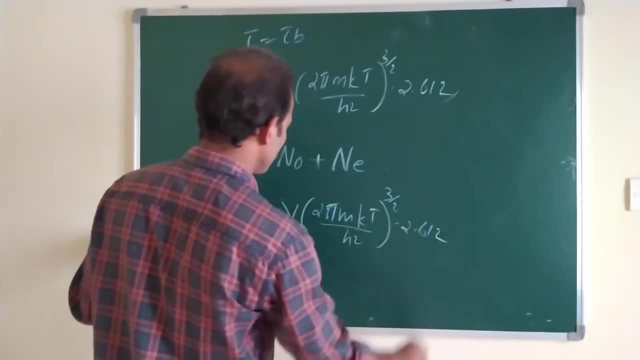 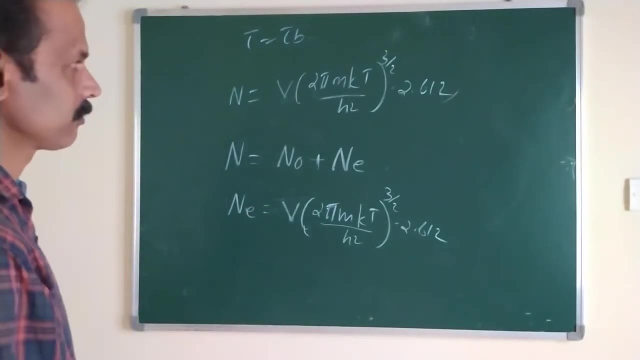 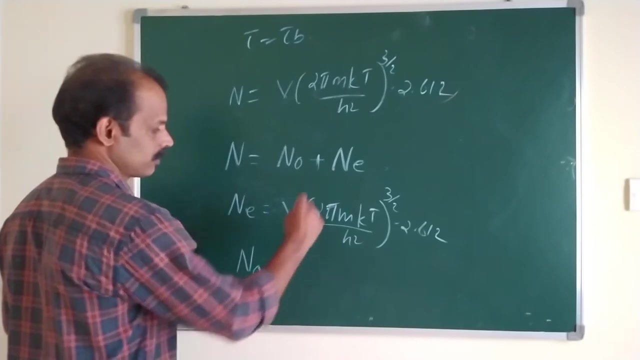 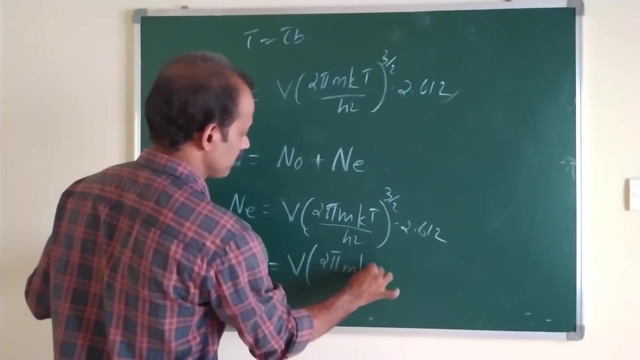 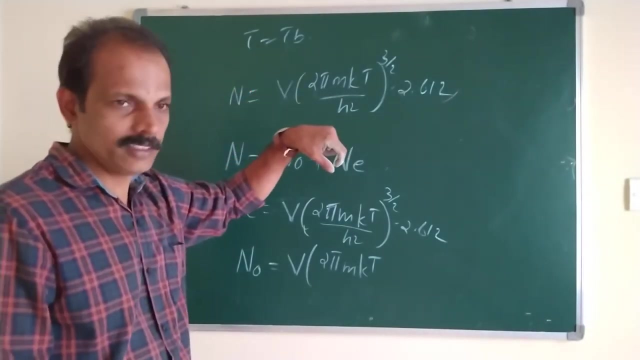 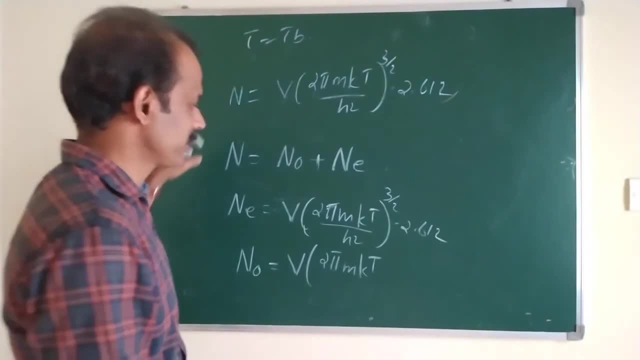 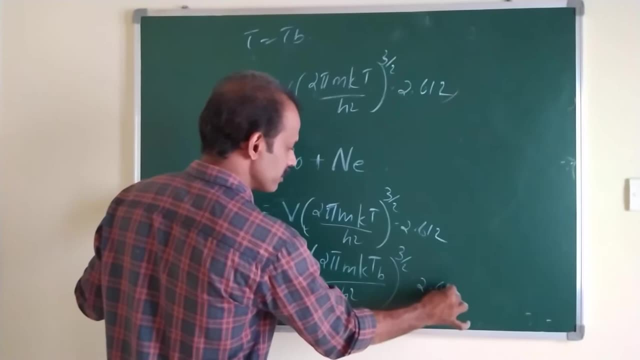 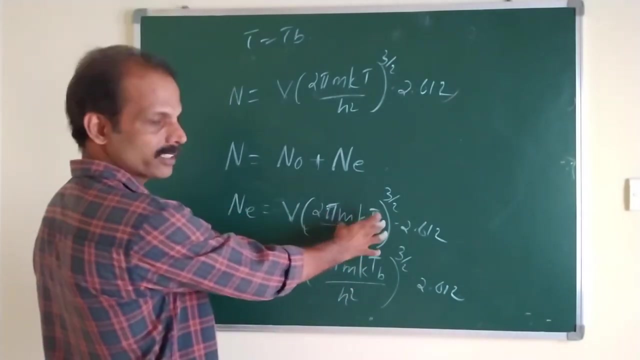 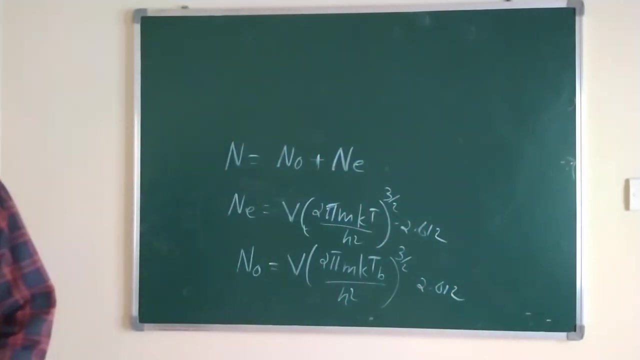 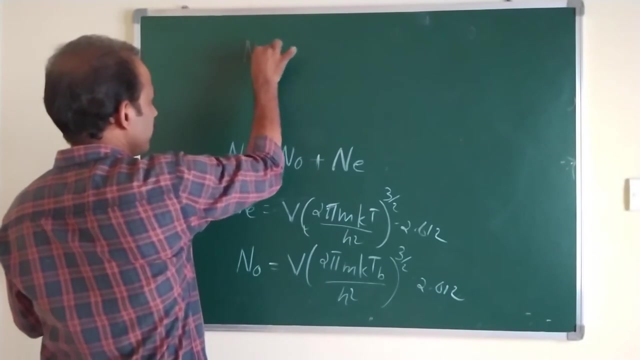 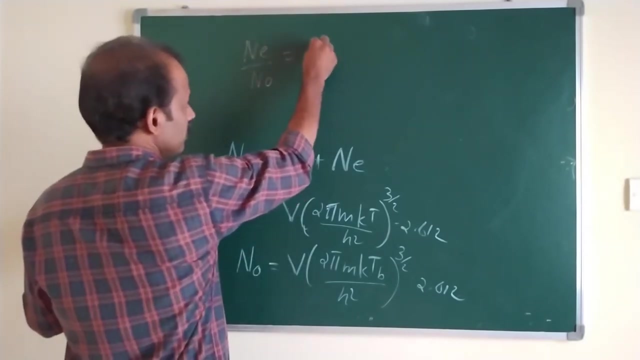 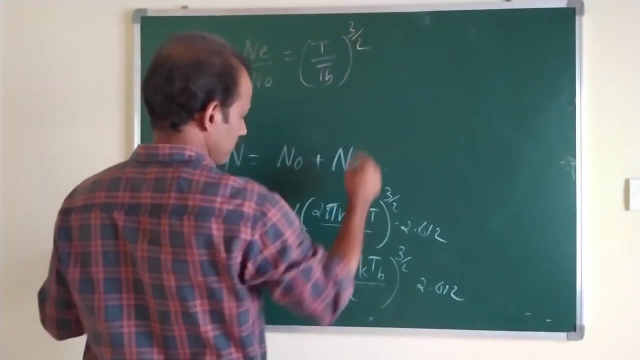 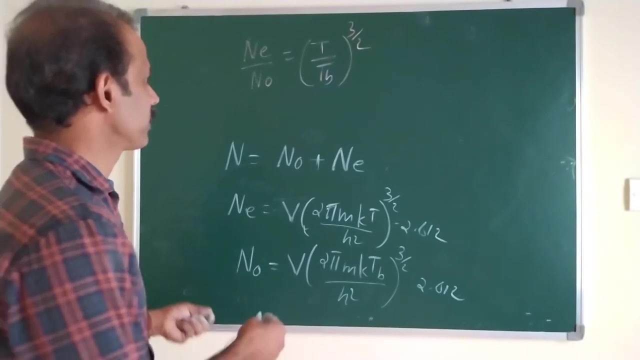 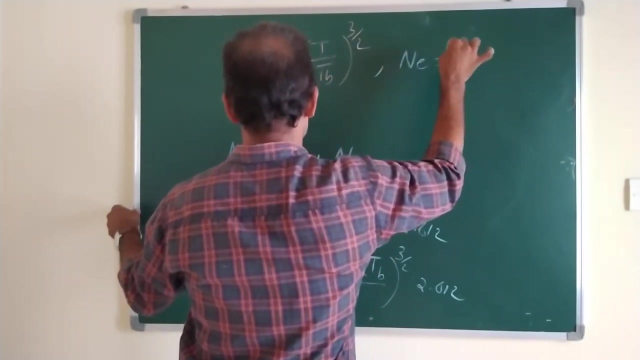 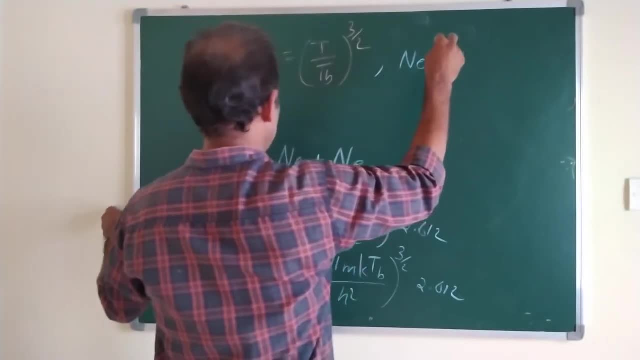 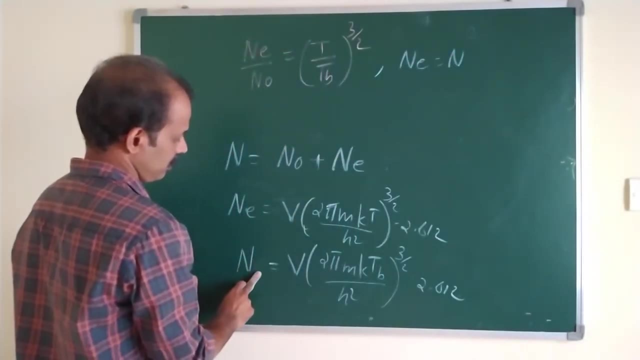 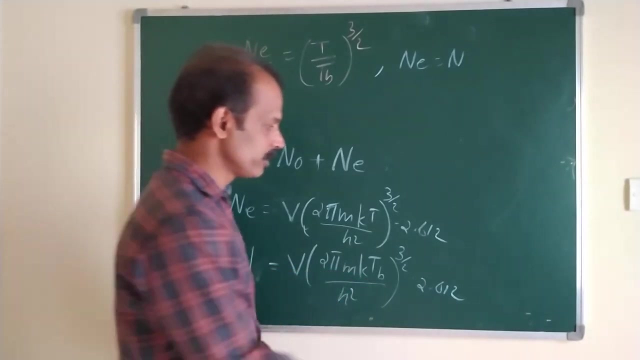 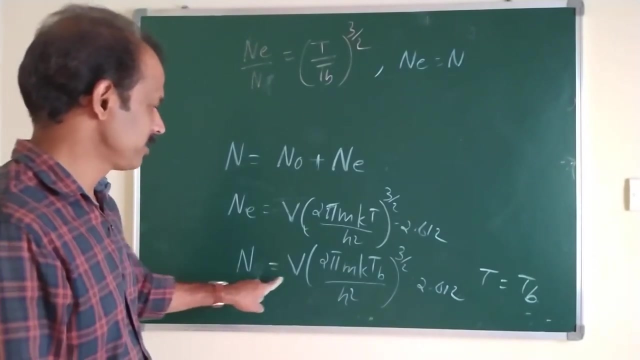 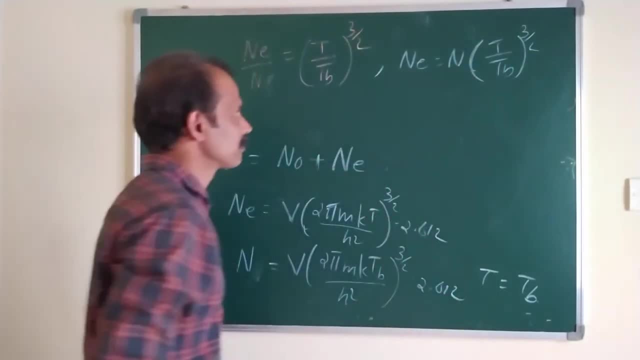 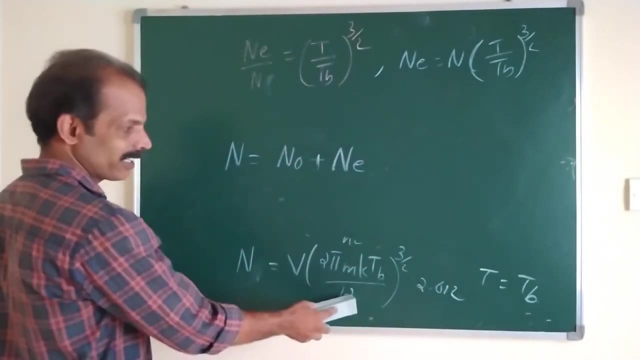 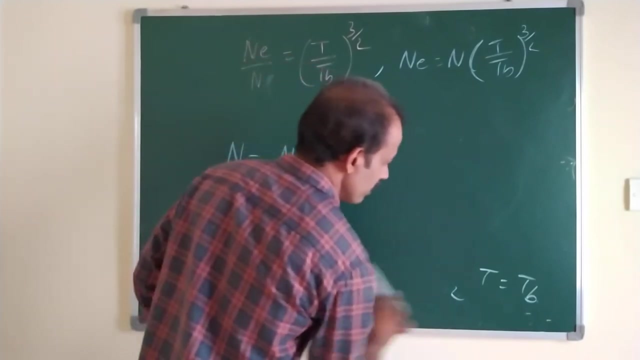 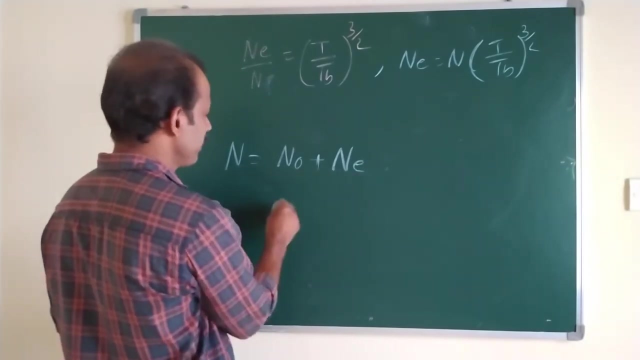 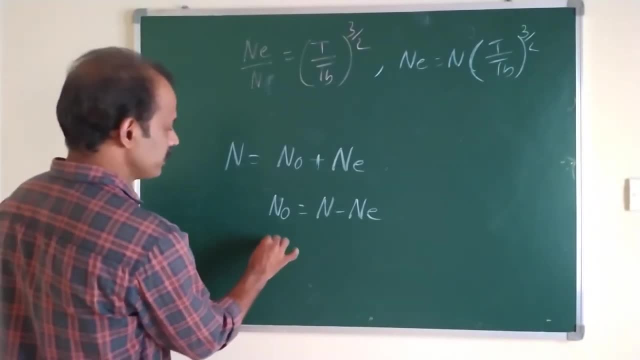 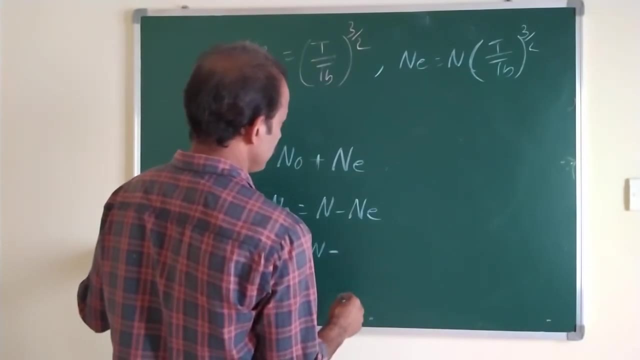 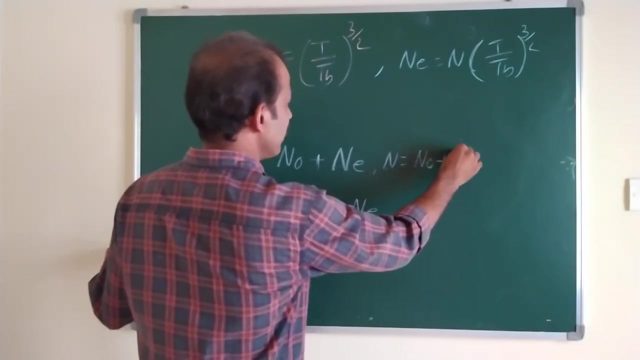 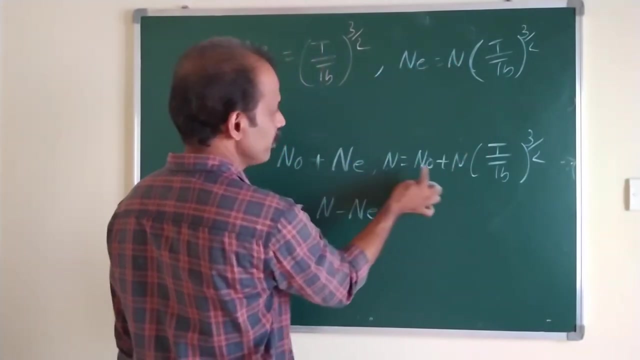 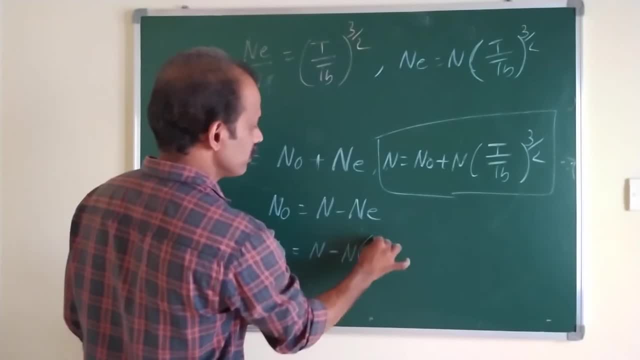 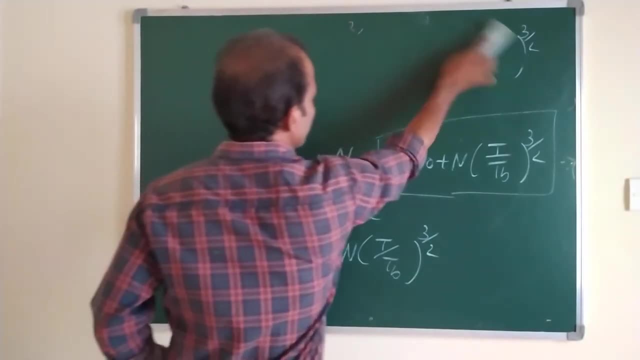 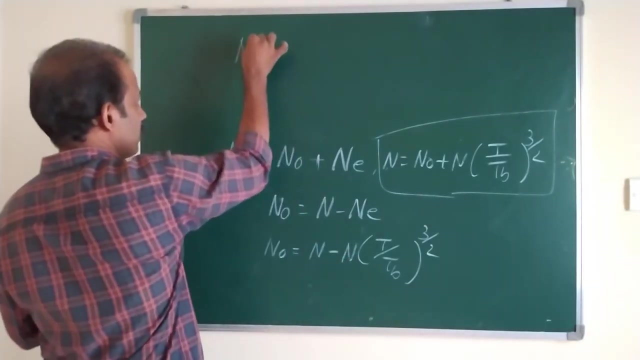 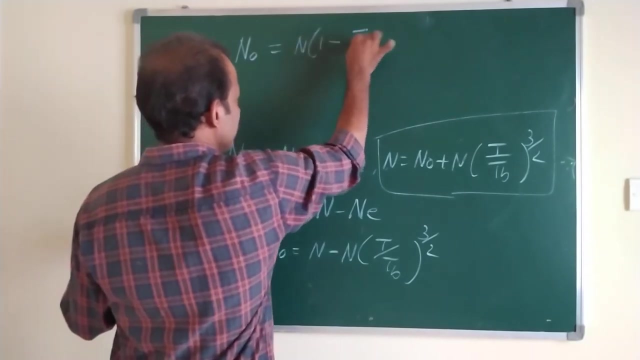 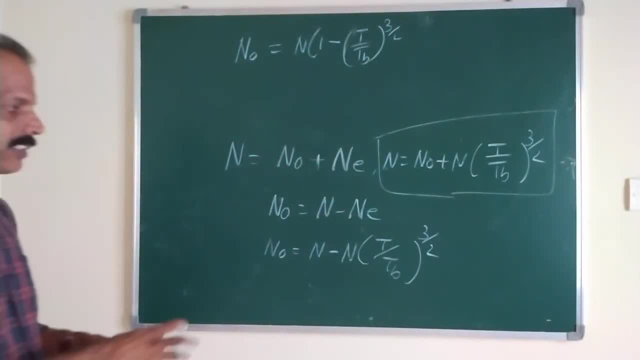 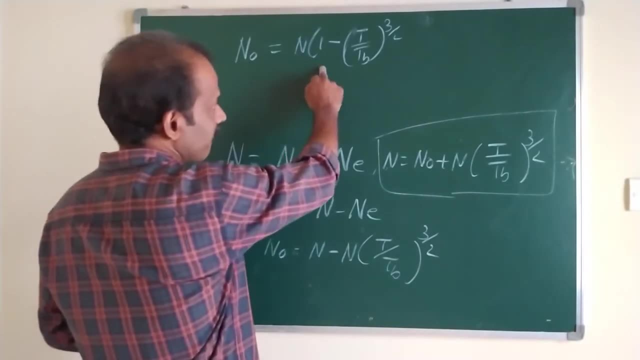 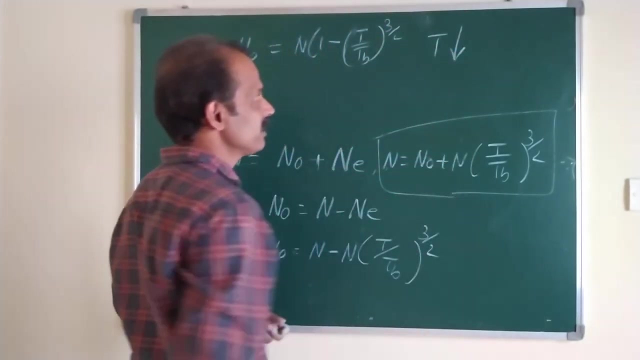 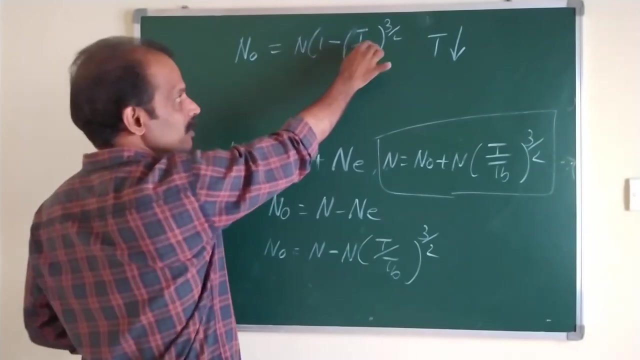 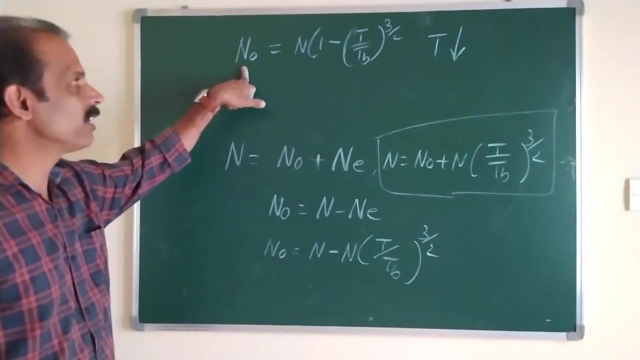 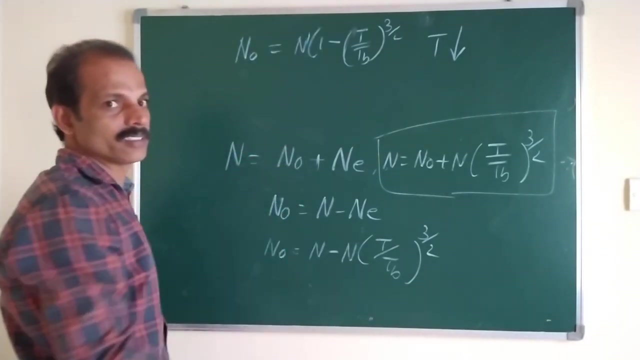 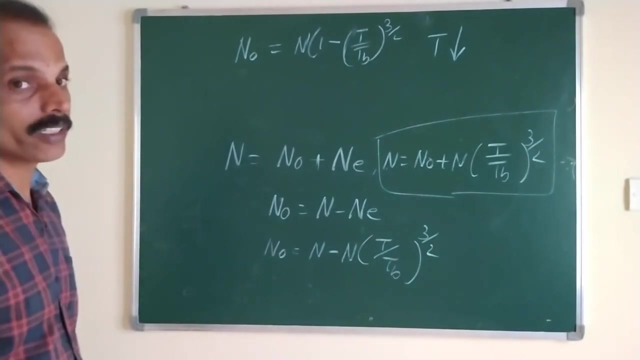 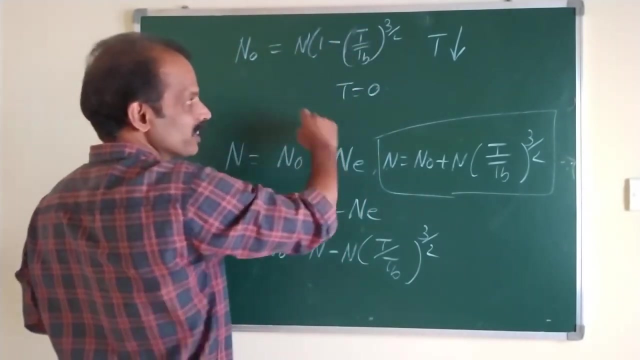 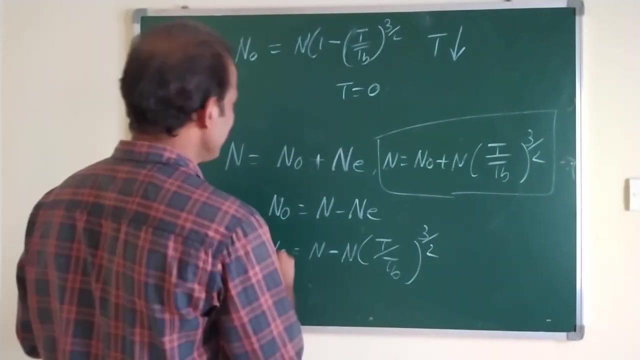 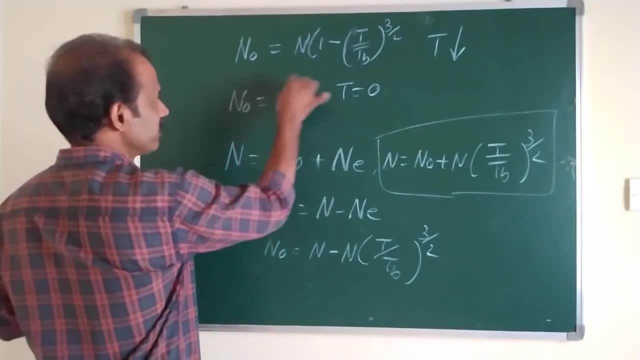 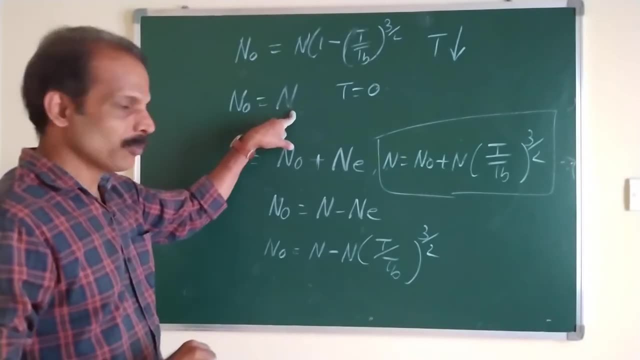 So what will happen? n0 is equal to n. This term will vanish. When it is 0,, this term will vanish. n0 is equal to n. What does it mean? This is the total number of particles and n0 is the number of particles present in the ground state. 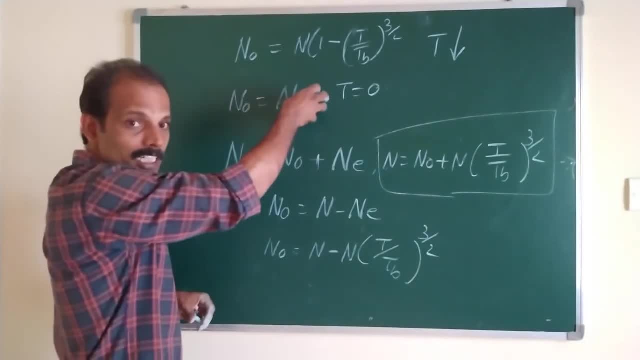 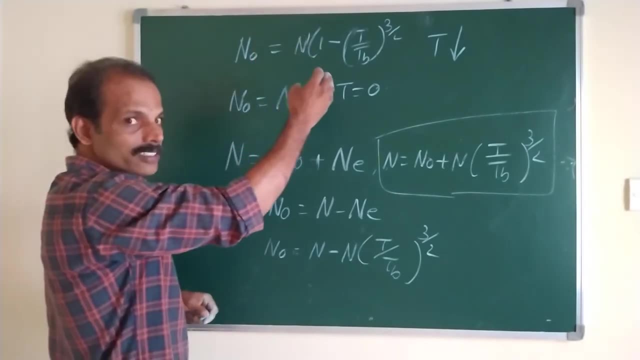 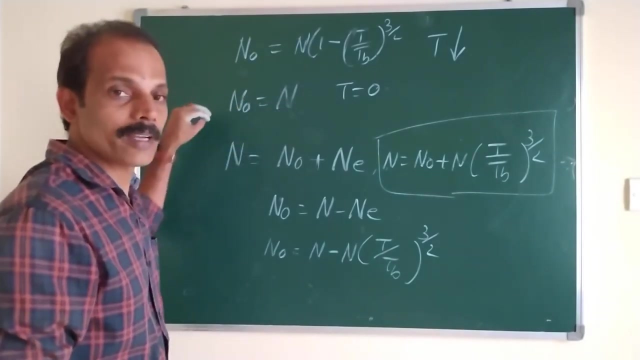 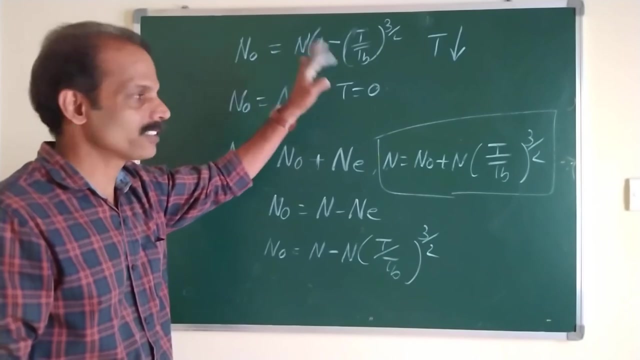 So all the total particles, all the particles present in the system, is equal to particles present in the ground state. It means all the particles comes to ground state and occupy it. All the particles, all the n particles, occupy ground state. No other states have any particles at. t is equal to 0.. 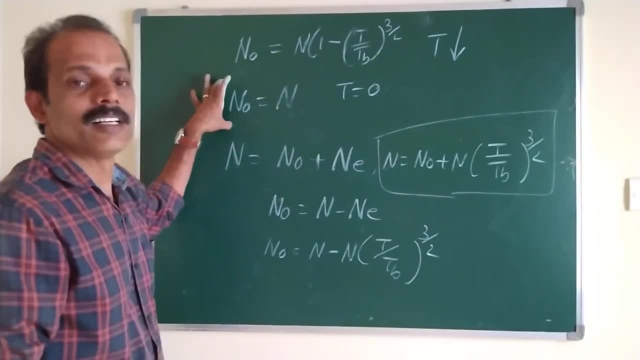 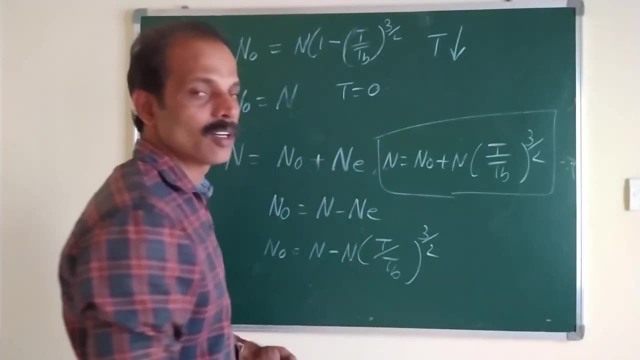 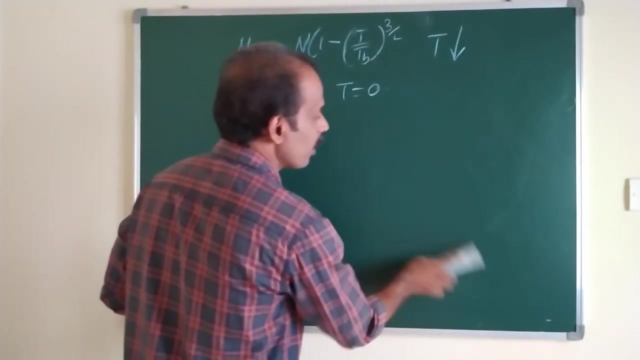 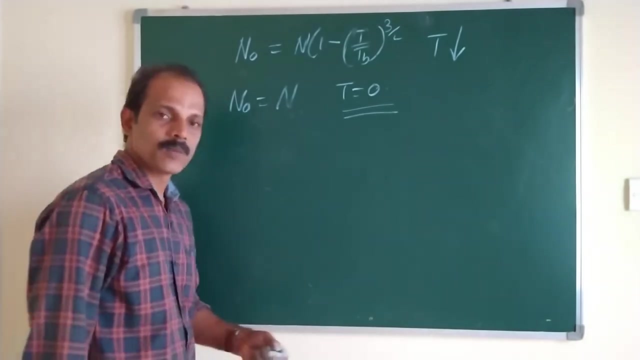 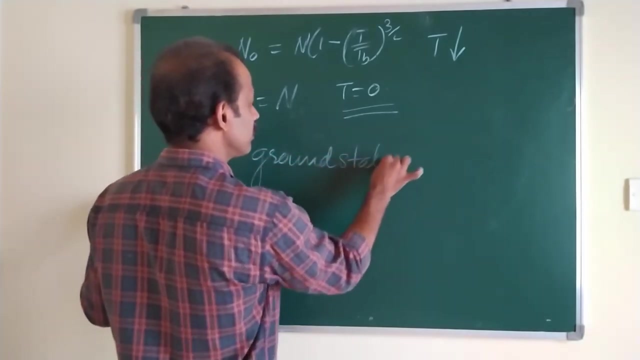 All the 100% particles will be occupying at a ground state that is n0.. That is what is known as Bose-Einstein condensation. That is, at t is equal to 0.. At t is equal to 0., All the particles of boson, boson gas, all the particles at temperature 0, all the particles of boson gas, will occupy ground state according to this equation.